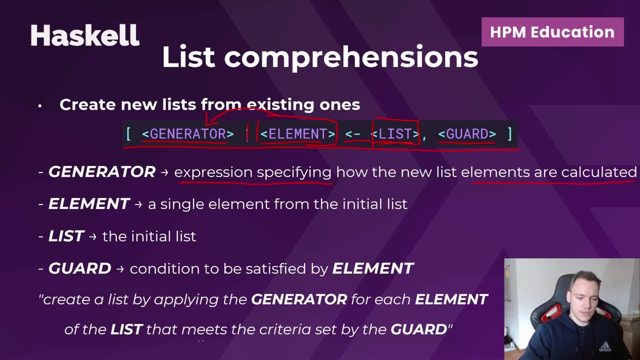 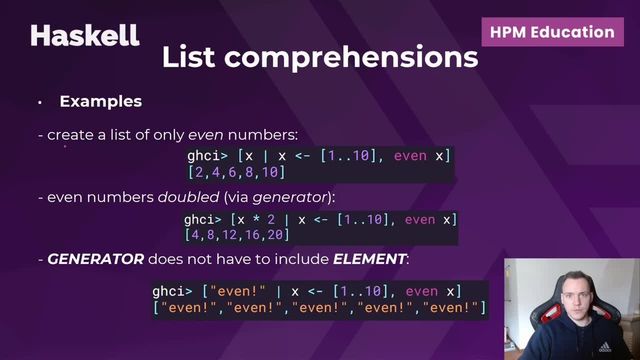 the generator for each element of the list that meets the criteria set by the guard. let's take a look at the generator. let's take a look at some examples of list comprehensions to get a better understanding. so in the first example, we want to create a list that contains only the even numbers. so we have an. 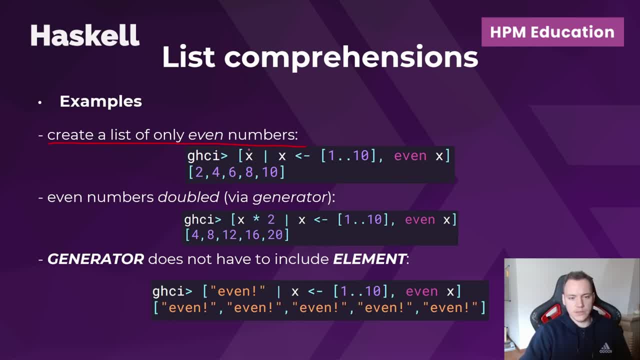 initial list and we want to take only the even numbers from that list. in this case we use x as the generator, where x is taken from this initial list that we defined here as the numbers one through ten, and then we have a predicate that the x element must satisfy to be pork. 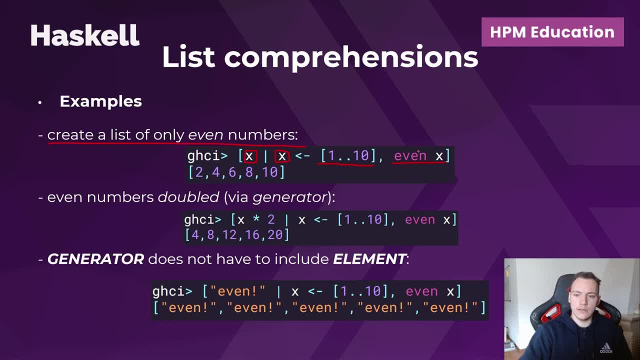 considered as a generator, and that's that the number x is even. so we apply the even function to x, and this guard always must be a boolean expression, so always must equate to either true or false, which is exactly what the even function does, and the result is a new list. 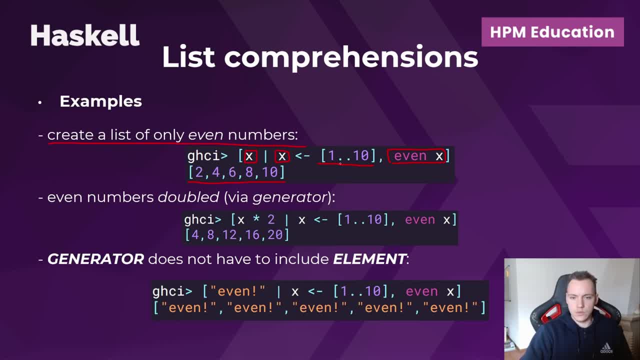 of only the even numbers from the first list, which was one to ten. Now we have only the even numbers from 1 to 10.. Okay, so the next example is pretty much the same, except I want to show here that we can. 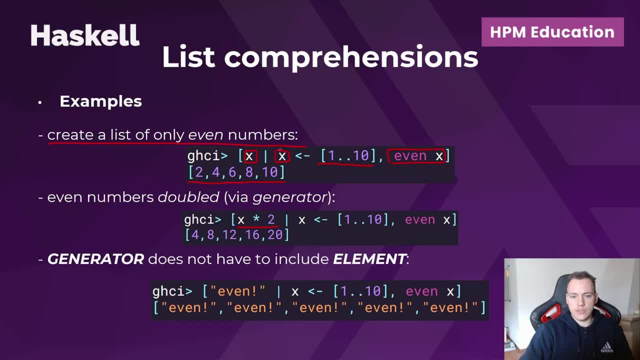 besides using the generator as is, as just an element from the list X, we can also apply functions to it to tell Haskell how to calculate new values for the new list based on the elements of the old list. So here we, for example, double all the even numbers. 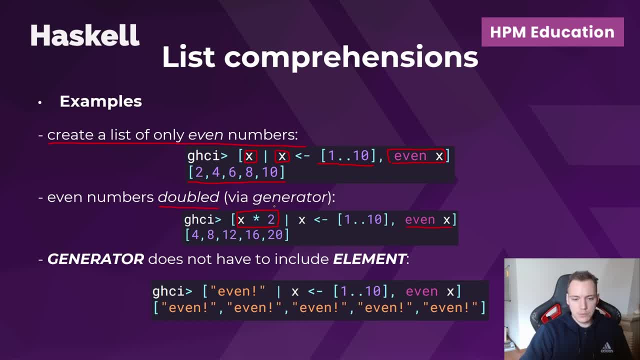 We still have the same predicate, so we check for even numbers, but in the new list we double each of them Right, so we can apply functions to the generator or in the generator clause. And the third one. the third example shows that generator does not have to include the. 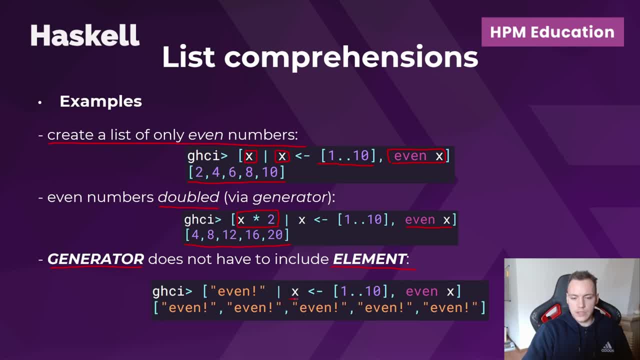 element. So we can just Okay, so we can just Okay, so we can just use the element as a checking of a predicate and we can create a completely- you know- different value for the new list. So, for example, here we in the generator, we just put a static value of a string, even. 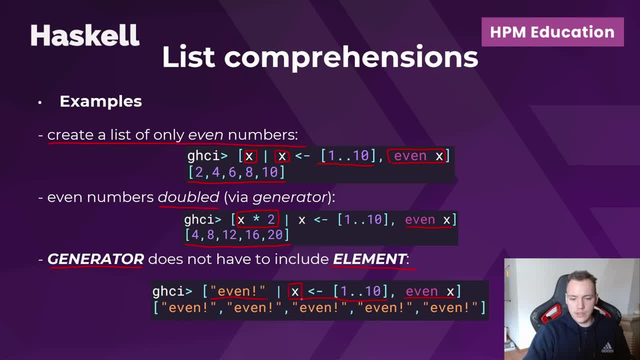 and if an element from this list, an element X, satisfies this predicate, then the generator will be triggered, and the generator will be triggered And the generator value will be included in the new list. So we'll have five of the same values in this case, and we do not use X as a generator at. 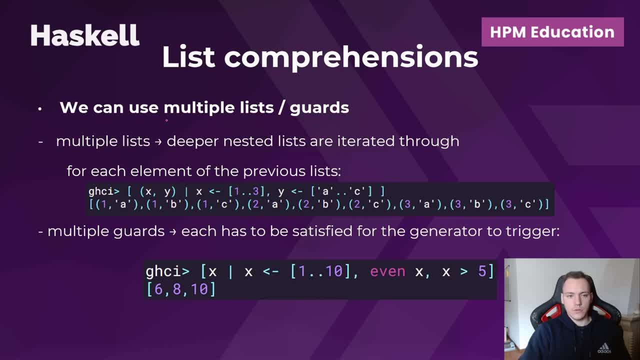 all List comprehensions are very versatile so we can work with multiple lists and multiple guards to create the new list. If we use multiple lists then the deeper nested lists in the definition will be iterated through for each element of the previous lists. 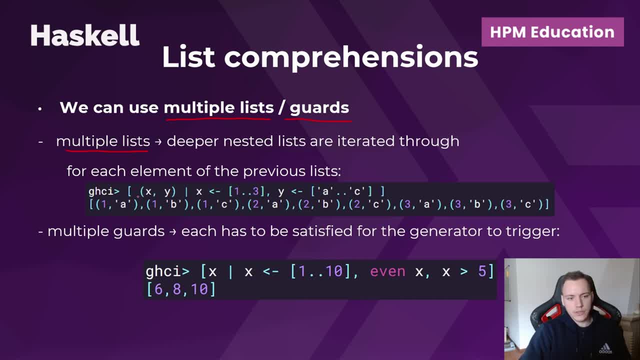 To show an example, here we have a list comprehension that generates a tuple value. okay, X and Y, where X is taken from the first list- one, two, three and Y is taken from the second list, from A to C, so ABC. 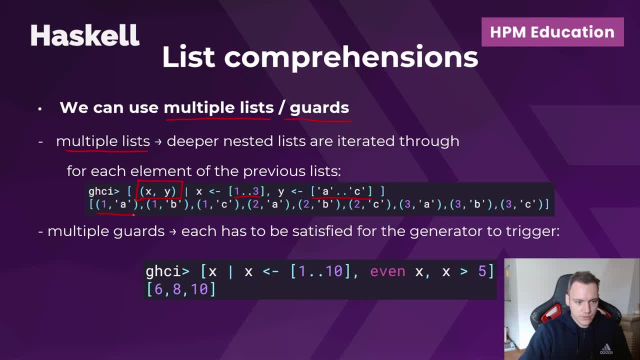 And we can see that in the result, the first three elements of the new list all have the same X value, One right, And the Y value is iterated through. so one A, one B, one C. Then for the second value of X, Y is again iterated through: two A, two B, two C. okay, 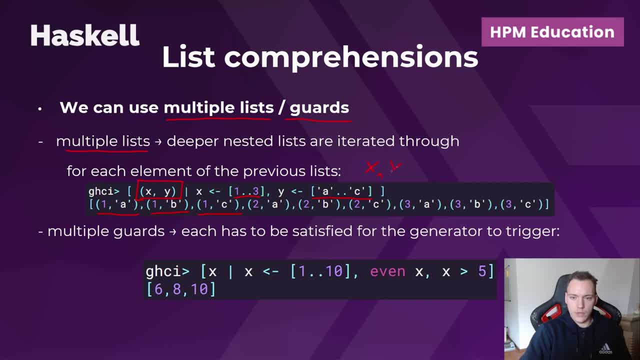 So the iteration goes as: X one, Y one, then X one, Y two, and so on. right, So the deeper nested list, Deeper nested being the ones further away, Okay, Okay, And the ones further to the right are iterated through for each element of the previous list. 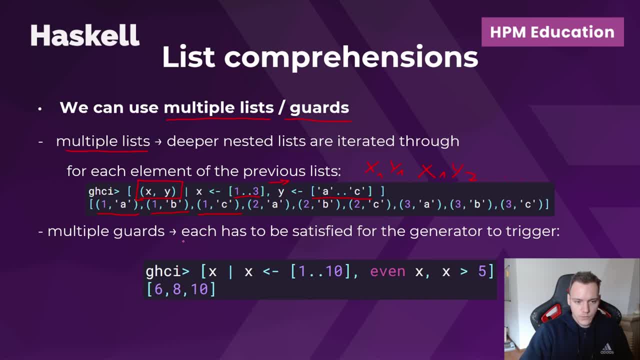 And with multiple guards it's simple. It's just that each has to be satisfied for the generator to trigger. So in this example we have the same even numbers list comprehension from one to ten. We check that the number is even, but we also check that the number is greater than five. 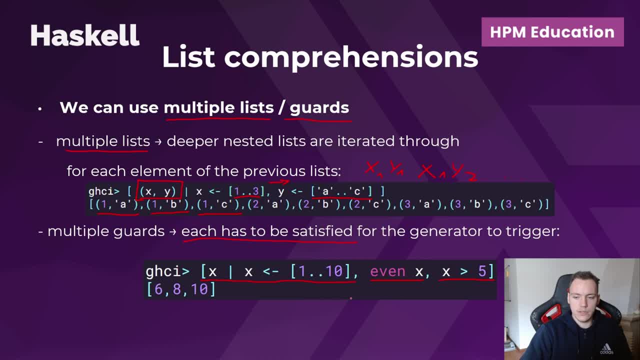 for example. So we have two guards and both of them must be satisfied For the generator to trigger, and in this case we only get the numbers six, eight and ten, as those are the only even ones and greater than five. 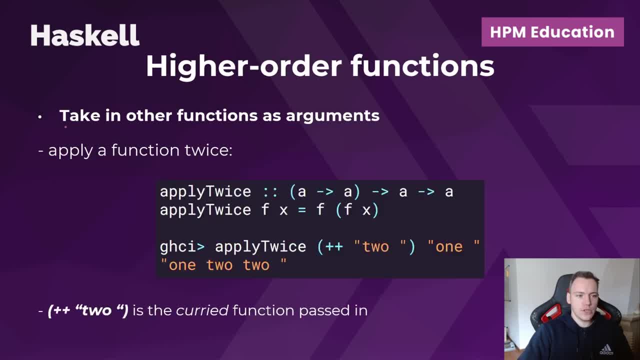 Now we get to higher order functions. So in general, higher order functions are functions that take other functions as arguments. So we already saw this in the previous video where we looked at the function operators and specifically The. The function composition and function application both accept a function as an argument. 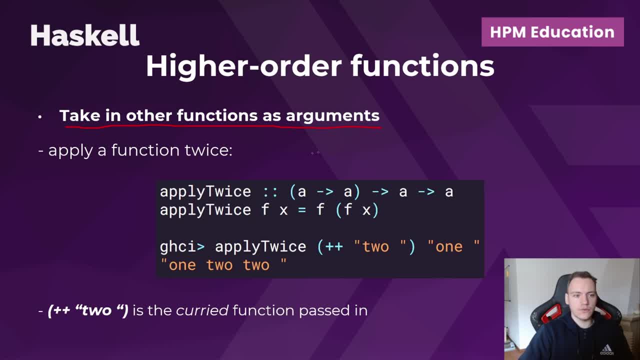 So strictly speaking they are also higher order functions. And here we have a function to apply a given function twice right. So to signify a function, as an argument we use the parentheses and then the normal function type signature. So from one type to another type, in this case, 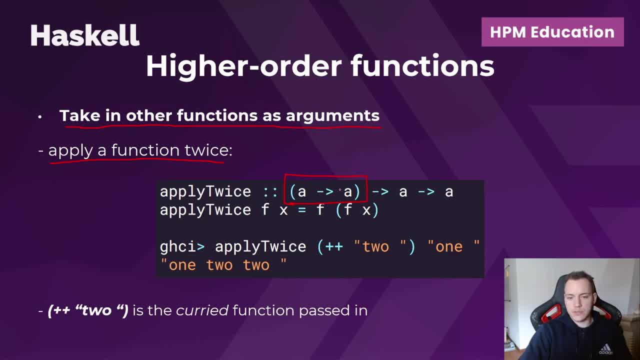 A to A And our function accepts a function that goes from A to A, accepts the argument A and finally applies this argument to the function, in this case twice, but in any case it produces again A. So the definition is apply twice. we accept the function as F. we accept the argument. 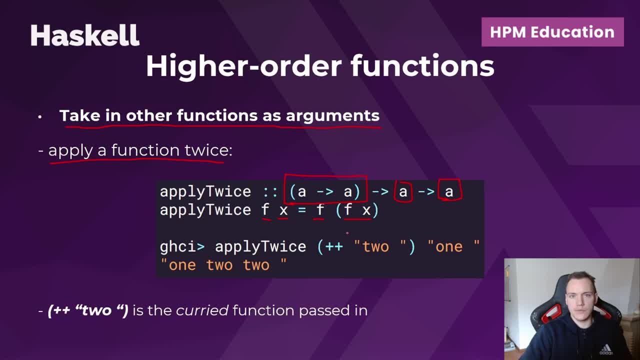 as X and we apply F to X and then again we apply F to the result of that application. So apply twice, And here we use partial application occurring. so with plus plus and then a string. We know that plus plus is the operator for list concatenation, so it takes in two lists. 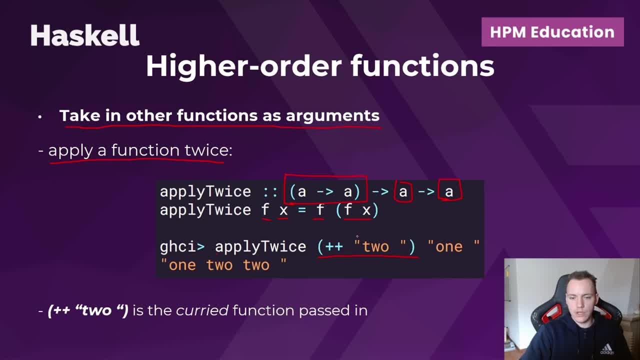 and returns their concatenation. In this case we apply it to only one argument, so it's a partial application. So this is a function. now, This whole thing is a function that accepts another function, Another list to join them together, And then we supply that second argument here and then this first function applies twice. 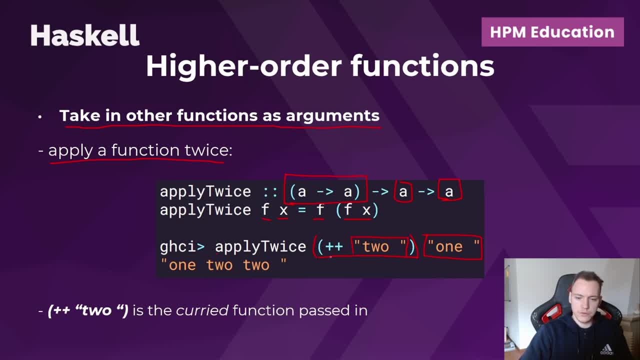 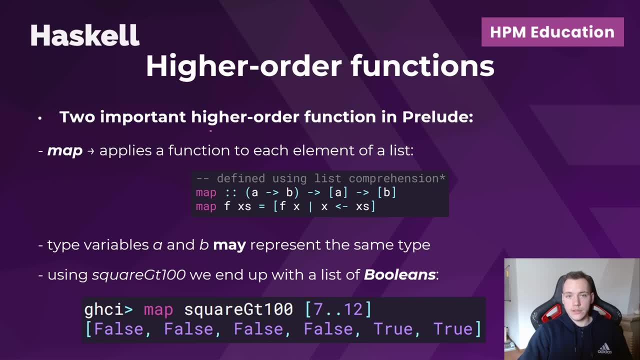 to it. So we have one plus plus two plus plus two. That's the result. Now we'll look at two important- or what I consider very important- higher-order functions in the prelude, The first one being map, which is, I think, the most important one. 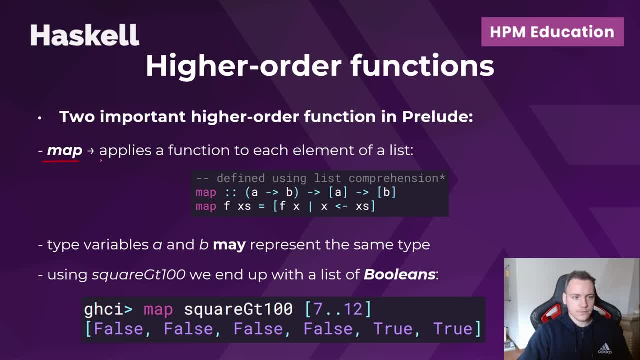 Yeah, And it's a function for working with lists, And what this function does is apply a function, so it's a higher-order function. it accepts a function and applies it to each element of a list. So, since we have just covered list comprehensions, we could define this function using list comprehension. 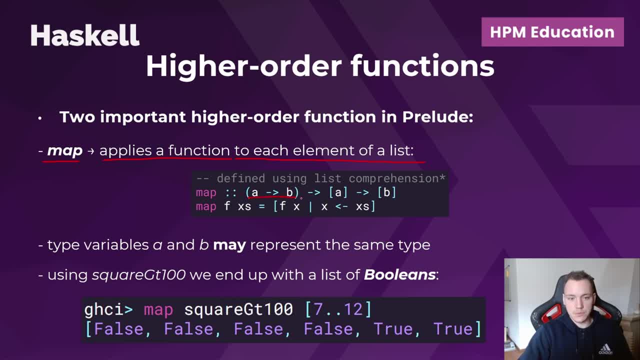 In this case, we know that it accepts a function. It accepts a list. Okay, So we have a list to apply that function to and it gives a result which is a new list with all the elements resulting from the application of this function to each of the elements. 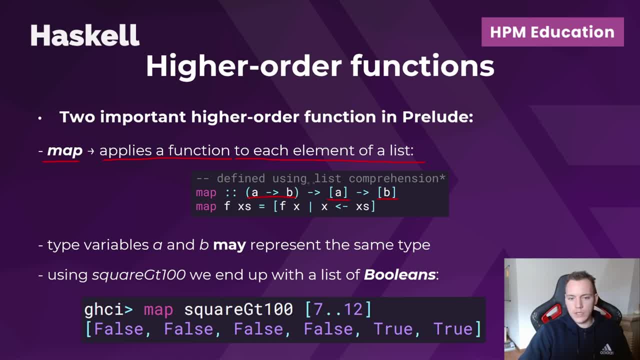 So the type signature says from A to B and then it accepts the list of As. so it has to be a list of As because the function accepts As as an argument and gives B as a result, And then we get finally a result as a list of Bs. 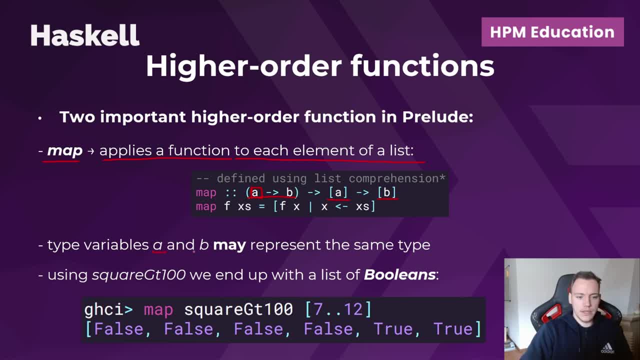 Of course type variables A and B may represent the same type here, because there is no class constraint. but it's just defined as polymorphic because we could go from, for example, a function could take in a number and return a string, and then if we apply this function to each 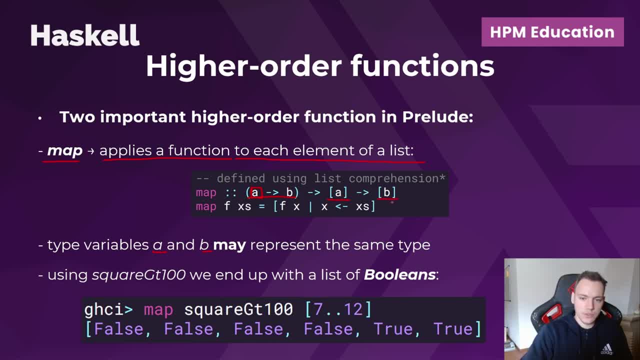 number in the list. we would get back a list of strings, So the types could be different, but again could be the same, Okay, Okay, So we define this with list comprehension. We take in the f as the function, we take xs as the list and we apply the function. 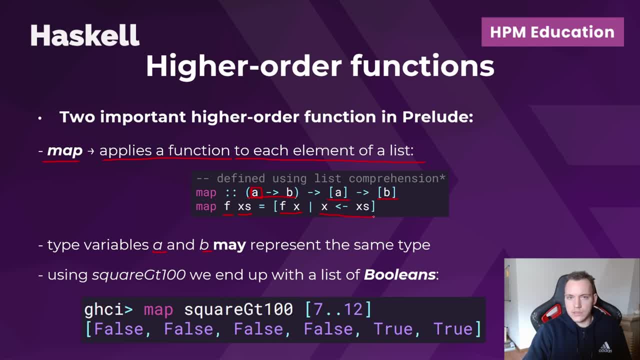 f to each element x taken from this list of xs. So if we take an example, with our square gt100 from last time, the function we defined in the last video, we end up with a list of booleans, right, Because this function returns a boolean. 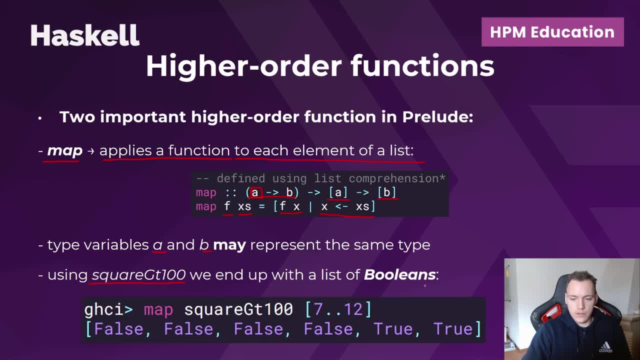 Either it's greater than or it's not, And then if we map this function to a given list, we get back a new list with the elements being the result of the function application. So square gt100 applied to 7 returns false to 8 returns false. 9 returns false. 10 false. 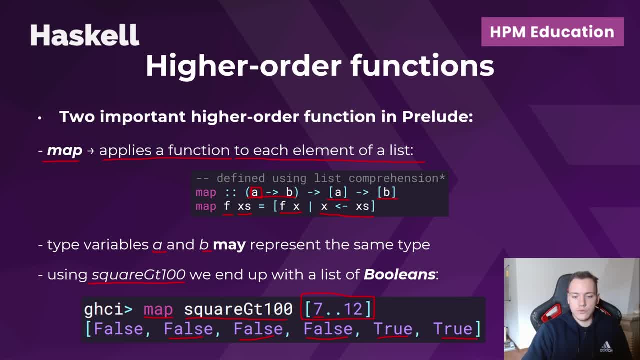 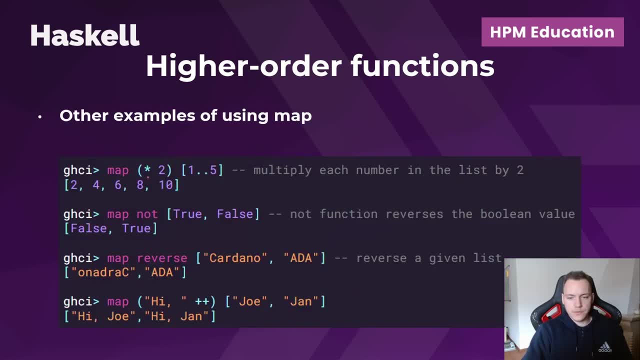 and then finally, 11 and 12 equate to true. Okay, Okay, So that's what we get in the new list. Here we have some other examples using the map function. So always, the pattern is the same. right, We accept a function and we apply it to some list or to each element of the given list. 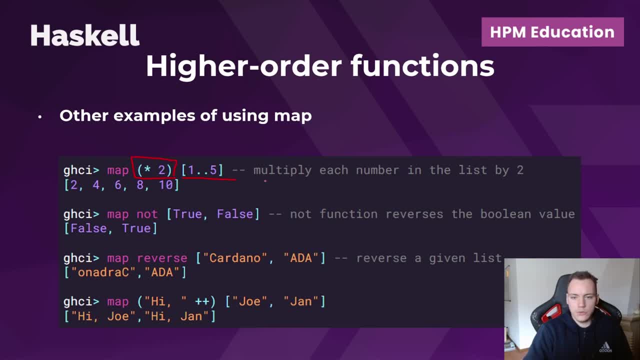 So in this case this function is multiplied by two. So every number in the list, one to five, is multiplied by two, We get back two, four, six, eight and 10.. Okay, We can map the not function which takes in a boolean value and reverses it, right? 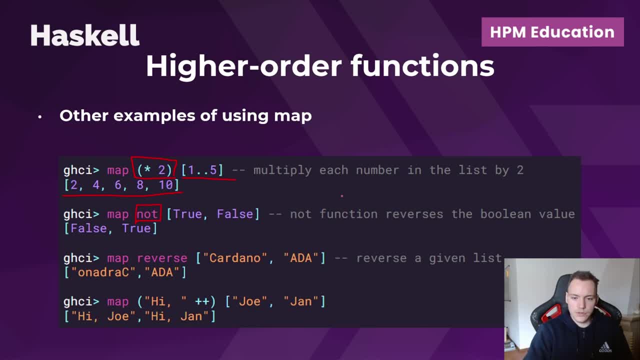 So not true is false, not false is true. So that's what we get in the result. We can map the reverse function that takes in a list and reverses the order of its elements. So we know that strings are actually lists of chars. 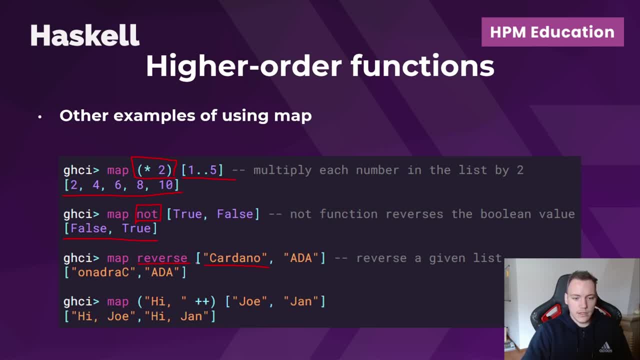 So this works with strings- and then each element- So not in this case, not the list- is reversed so that we have Ada and Cardano, but each of the elements is reversed because map applies this function to each of the elements. So, reverse, apply to Cardano and apply to Ada. 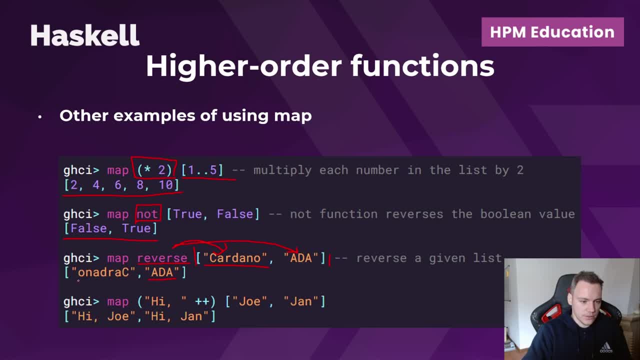 Of course, with Ada it stays the same because it's the same order, but the Cardano string is reversed here. Okay, We can also have some function. This is again using partial application of the plus plus operator, And then we apply it to the function to concatenate the strings. 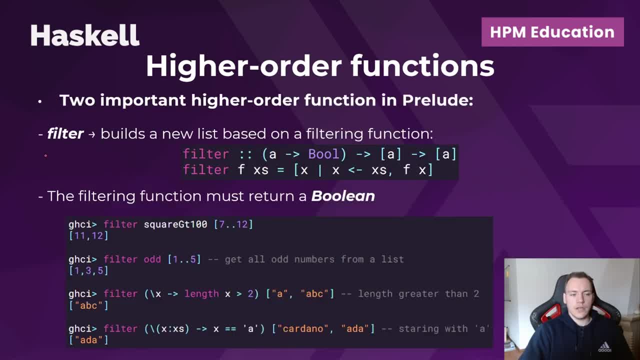 So we get hydrohygen. The second function I wanted to mention here is filter, which is also another higher order function that works on lists And it builds a new list based on a filtering function. So the higher order function in this case accepts a function from A, which is the type. 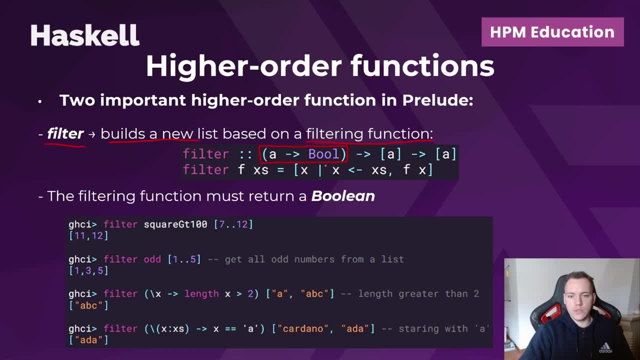 of the element in our list and returns always a boolean value. as a result, And if this boolean is true, then this element will be in the filtered list. If it's false, it will be discarded. Okay, And then we give it our list of As. 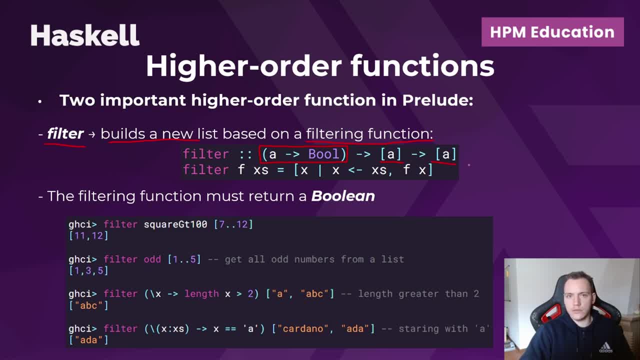 And we get back a list of, As The same type, only certain elements dropped which don't satisfy the predicate or the filtering function. right, So we can also define this function with list comprehensions. We take in the filtering function, we take in our list as XS and now our list comprehension. 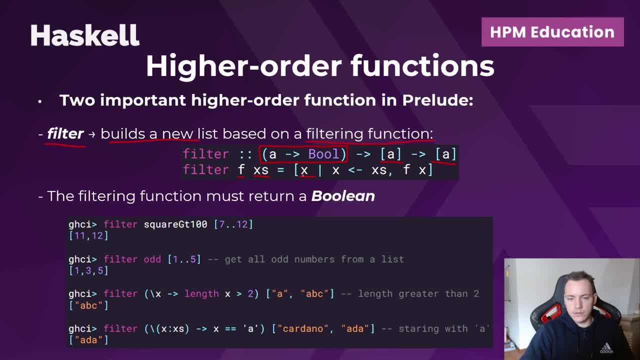 will take the value X in the new list where X is taken from this XS list, But only if the application of the filtering function to X equates to true right. So that's the filtering function And we can check some examples here. 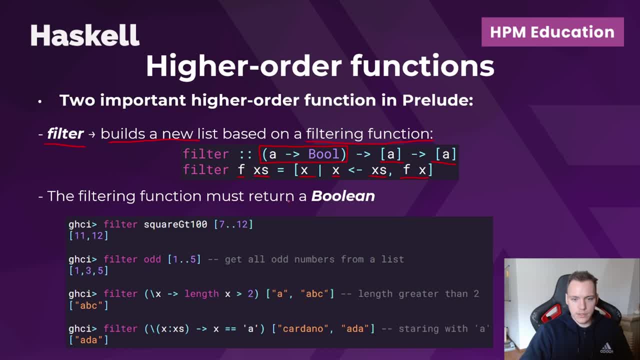 So the important note is that this function that we take in always must return a boolean to be a valid filter, unlike map. If we filter square GT100 on this list, Okay, Okay, Then we remember that 7,, 8,, 9, and 10 are going to equate to false for this function. 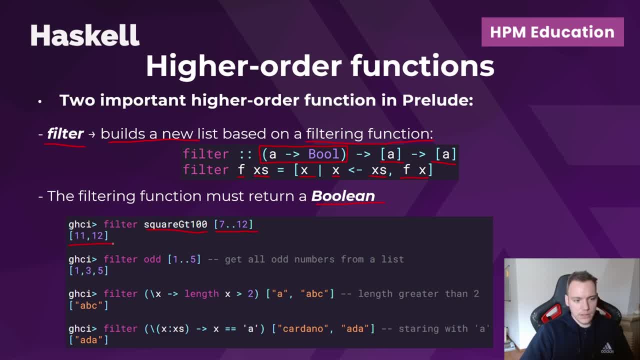 So those elements will be dropped, And then we only get 11 and 12, which satisfy this predicate. We can also filter out using the odd function to get all the odd numbers. So we get 1,, 3, and 5.. 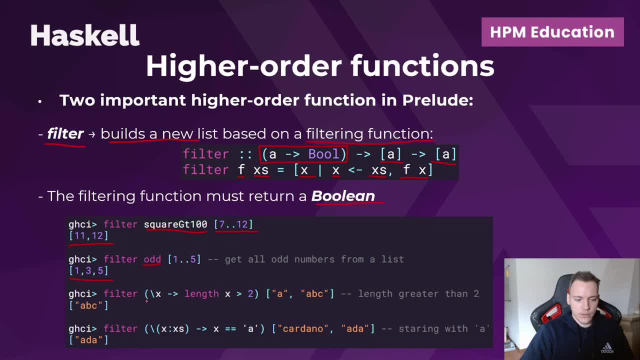 We can use lambda functions as the filtering functions, Because they return a boolean. So here we have a lambda function that takes in an argument X, And the function body is defined as if the length of X is greater than 2, then it's true. 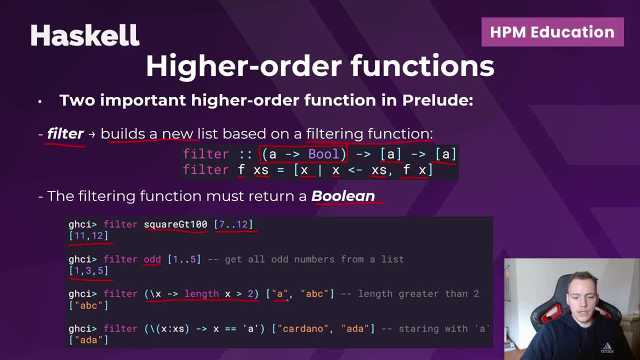 And if it's not greater than 2, it's false. So A- the length of this is 1. It's false, And ABC the length is 3.. So this is true And in the new list we get only the ABC string back. 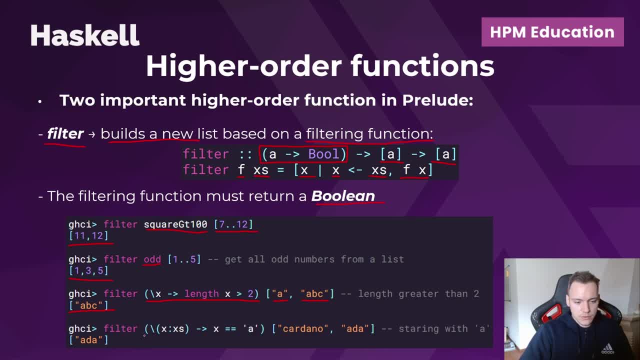 So here is another example of using a lambda function and the pattern matching of X, X, S, Where we take this pattern and we say: if X, if the head of the list is equal, equal to A, then that's the predicate, right. 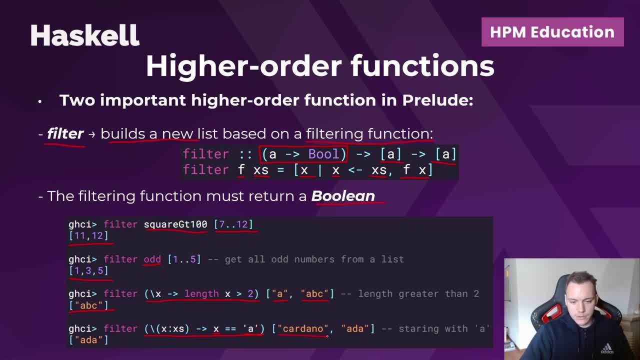 That's true, And if it's not, it's false. So in our Cardano ADA list we only get back ADA in the new list, Because ADA starts with A and Cardano starts with C. That's the end of this presentation. 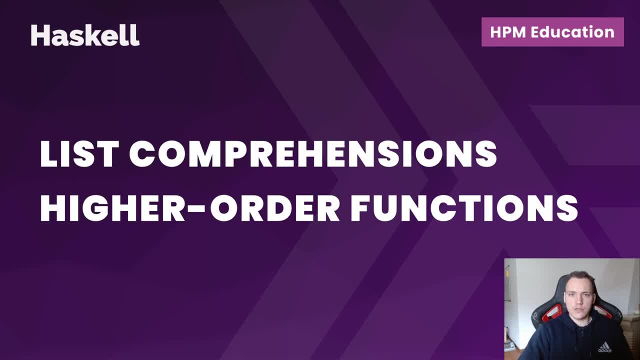 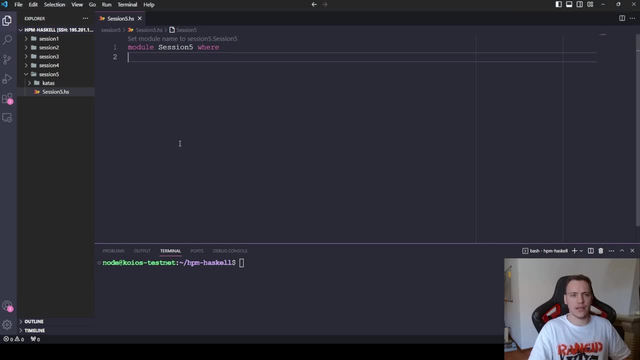 We covered the basics of list comprehensions and higher-order functions And now we'll go into the practical part where we'll try to solve some examples using these concepts. Let's start with list comprehensions. So we said list comprehensions are a way of defining lists in Haskell through existing lists or other lists in Haskell. So we said list comprehensions are a way of defining lists in Haskell through existing lists or other lists in Haskell. So we said list comprehensions are a way of defining lists in Haskell through existing lists or other lists in Haskell. So we said list comprehensions are a way of defining lists in Haskell. 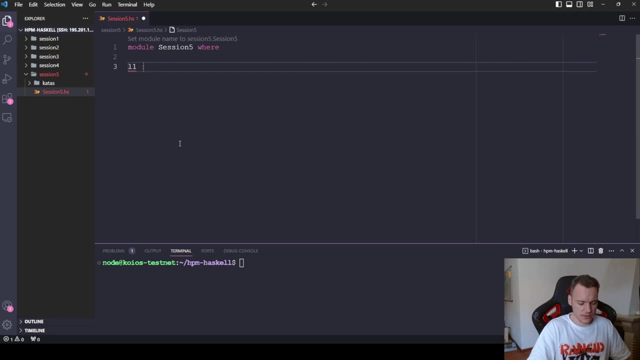 So we can define here a static list. Let's call it L1.. And it will have a type of integer And L1 will simply be a list of 1 to 5.. And now, for example, let's use the example from the presentation that dealt with even numbers. 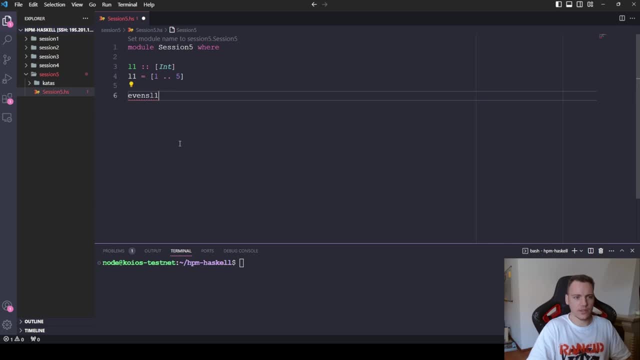 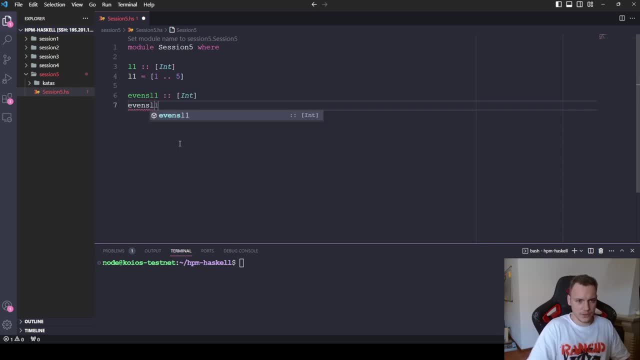 So if we want to say evens of this L1 list, it will also be a list of integer And we will simply define. So what we want to define is a list of even numbers created from this list L1.. So we can use the list comprehensions. 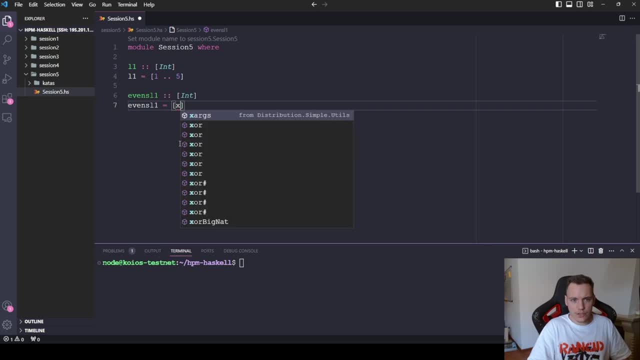 And the syntax is the generator. In this case I'll call it x- Then from which lists the x is generated. So we have: x is taken from the list of xs. In general, this is the pattern, But here we can use our static L1 list that we defined here. 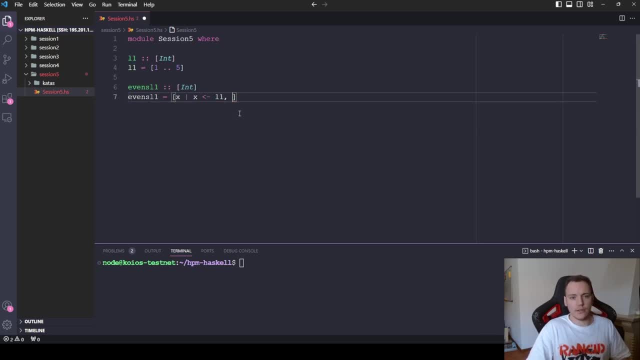 So it will be available here. And then, lastly, we could have another list here, More lists to generate new values from, But here we don't want to, We just want to end it with a guard. That is a predicate that the generator must satisfy. 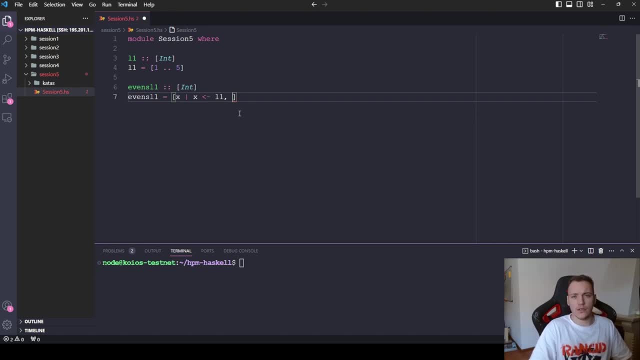 The element from the L1 list must satisfy In order to To end up in the new list. So in this case this is simply even x. The number must be even Right. So we can check this in GHCI If we load our. 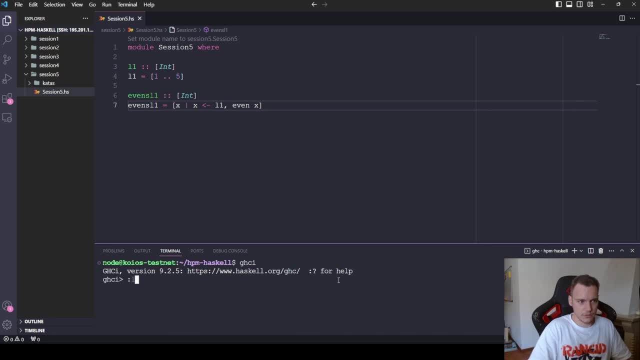 Where am I Load session 5. Session 5: HS. And so we can. We have access to L1,, which is simply the list, And we have evens from L1,, which is just 2 and 4.. Let's do one more example of list comprehensions. 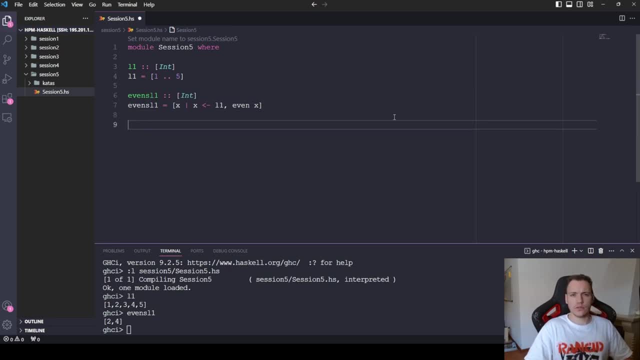 Say, a function that counts the number of times a character appears in a string. Okay, so we'll call this function count, And it will accept a char, a character, It will accept a string, a list of characters, And it will give back an int, which is the count of the number of times that this character appears in the string. 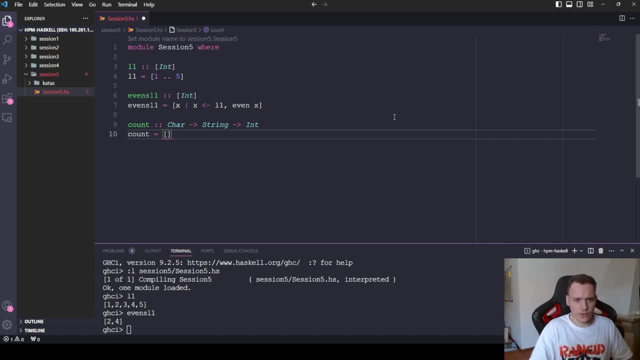 Okay, so we want to use list comprehensions Or list comprehension, And what do we want to do? We would like to first create a new list that contains only the characters of the previous list That match our character, right? So we have two arguments here. 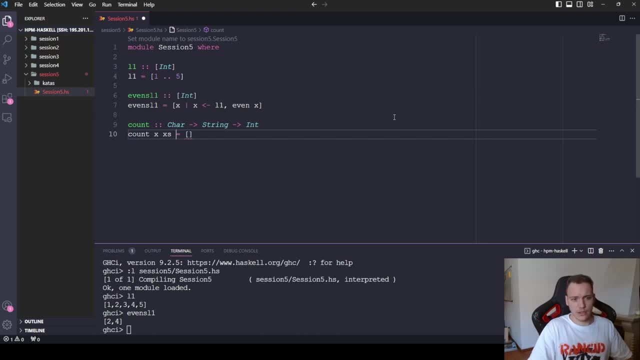 The char argument, which we'll call x, And the string argument, which we'll call xs, right? So if we create a list, a new list, of multiplied characters x, We could do that as, So we cannot use the generator x. 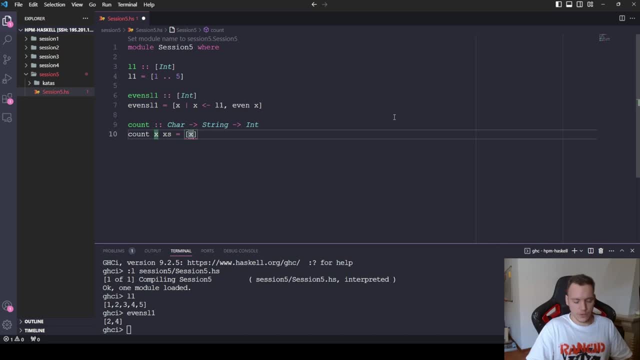 Because that's the name of the argument already. So we can use x' And so x' will be taken from the list xs And it must satisfy a predicate, right? We only want to take the character from the list if it matches the character we are looking at, right? 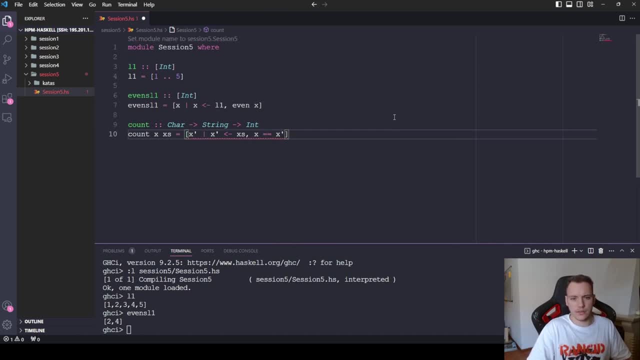 And that is x. So x must equal x' Now I'm not sure if, Okay, this is Right. so it says couldn't match expected type int. right, Because our function should return int. But this is a list of characters as it is. 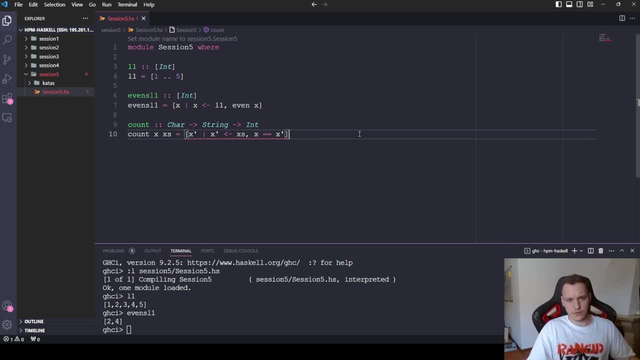 So, basically, we took all the characters that match our character we're searching for, And we have a new list of just those characters. So we simply need to check the length Of this list to know how many characters there are in there. Okay, so let's test this out. 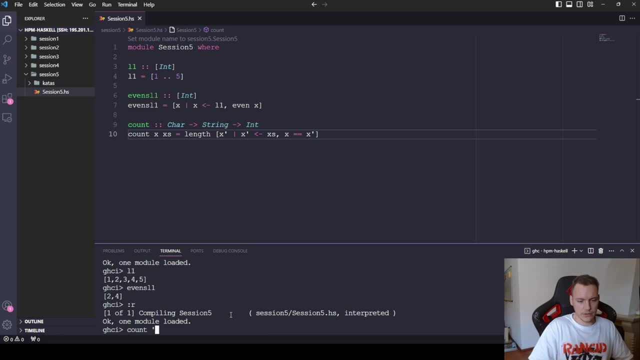 For example. so we have count, And then we have a character. Let's call, let's say s, And how many times does s appear in success? Three times, Okay, so that seems correct. Note that we didn't do any. 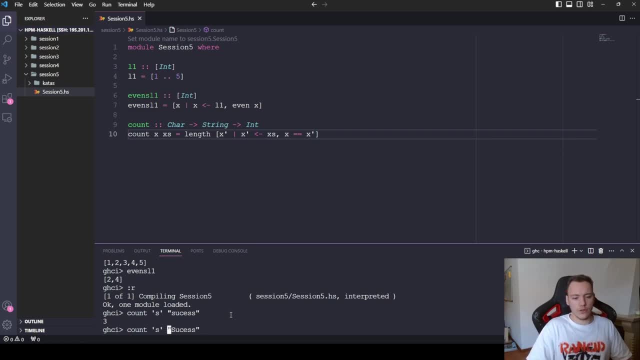 Too lower or Or something. So lowercase s is not equal to highercase. So we capitalize our list. We'll get back the count two right, And if we search for the capital S, we'll get back one. So we just look at the exact character. 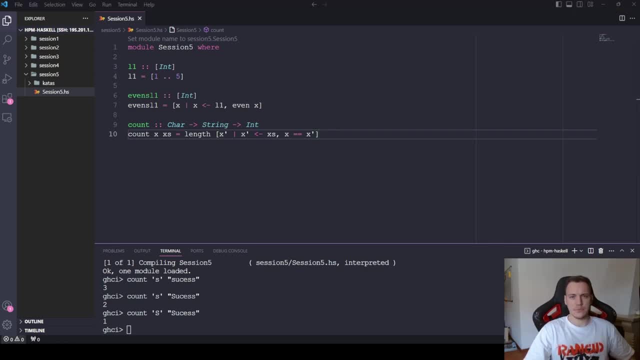 And it's case sensitive in this case- Besides list comprehensions, we also learned about higher order functions, And specifically two higher order functions- Map and filter For working with lists. So we had some examples of map for, Such as, multiplying the numbers in a list by two and so on. 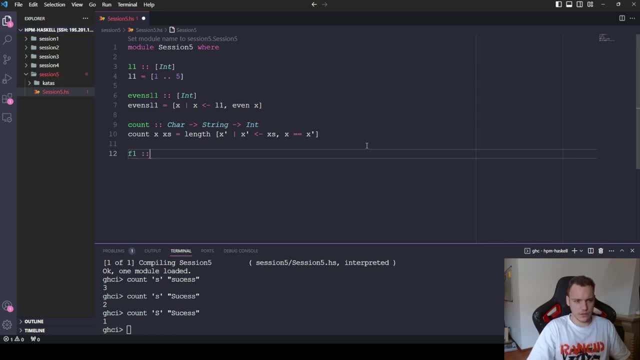 Let's write some functions, then here I'll just call it f1.. And that will be just a static value of integers. So the example from the presentation was So if we map And remember, we can check the type, signature of map. 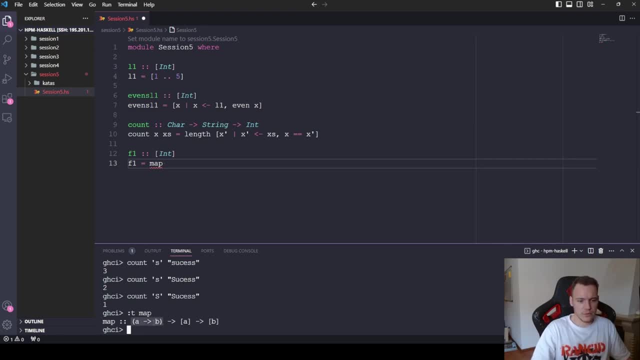 So higher order function accepts a function as an argument. A function from A to B Accepts a list of A's and returns a list of B's. So it applies this function from A to B to each element A of this list To return a new list with values generated from the function application. 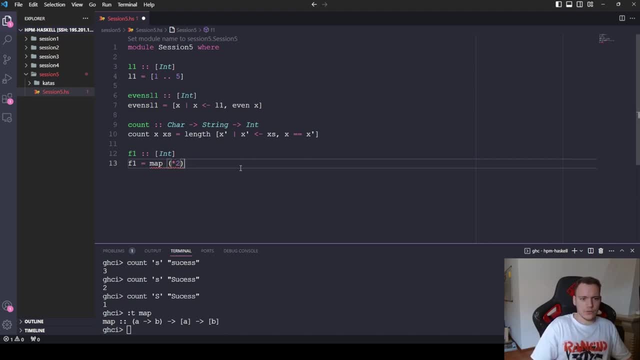 So we can use curring To do multiply by two And then apply to a list of one through five. And now this: all the elements in this list will be multiplied by two For this expression f1.. So we get two, four, six, eight and ten. 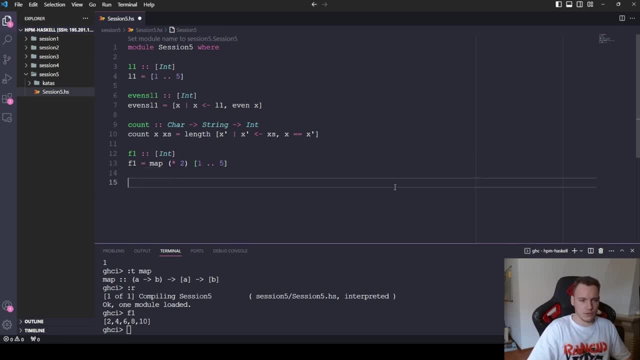 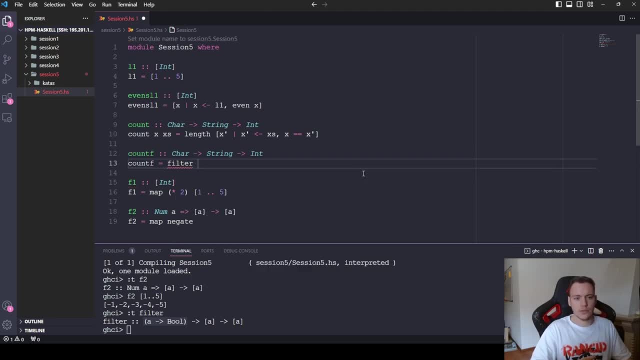 So we can also map other functions of course. For example, there is a name, So we have Filter and then our function that we. this function will still be applied to each element and if the element, if the function application to the element, results in true, then that element will be included in the filtered list. 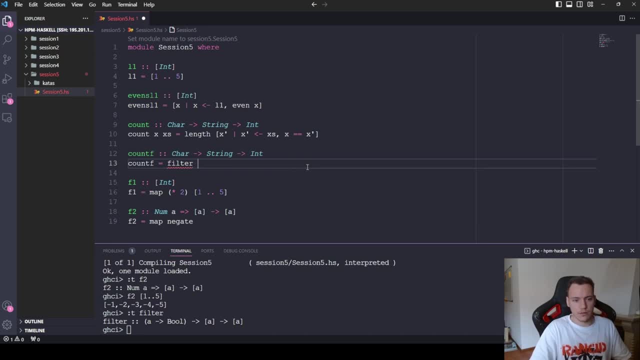 If it evaluates to false, then it will be excluded. So our function that we want to use is that, and we'll use Curring here. So let's have the same argument. So let's have the same argument. So let's have the same argument. 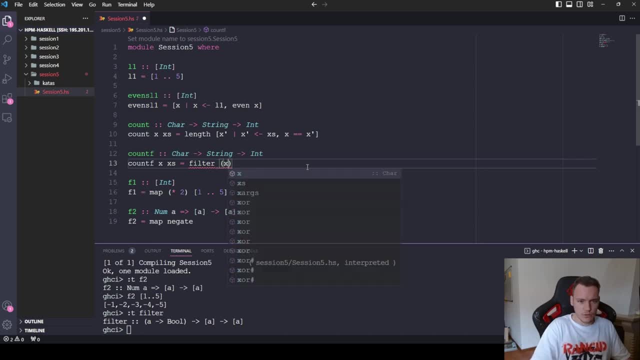 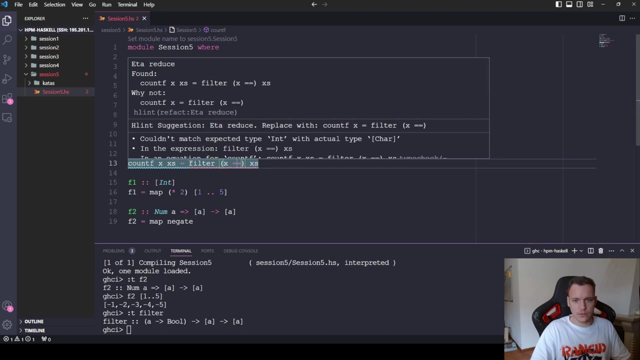 names for count f, so x and xs, and what we want to check is that x is equal, equal right. so to each element we want to apply this function: x equals the element of the list, and then we apply that to xs and i think that should be fine. okay, so of course the type is not right because we 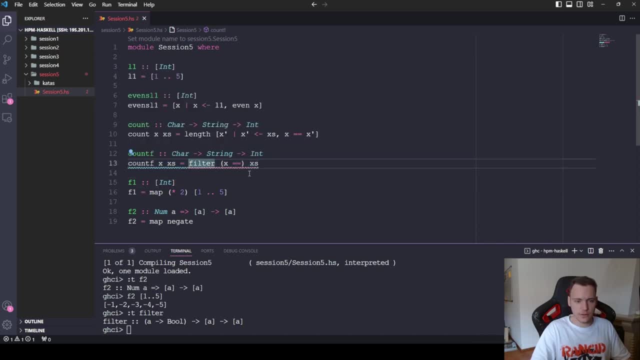 expect the type int, but this is just a filtered list. so we put this in brackets and then use again the length function and now we should be fine. so if we reload and then we say count f of the character s again in success, we get back three as well. so this is an example. 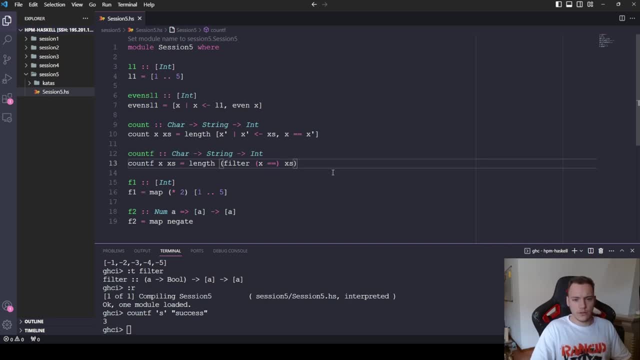 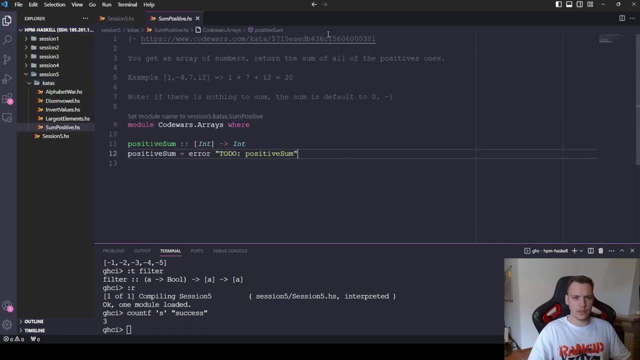 of you of using the filter function instead of list comprehensions. okay, now let's get into the katas. for this session, i prepared five of them and we'll start with this one. sum positive. i think it's a simple one to start with. this function should work the following way: you get: 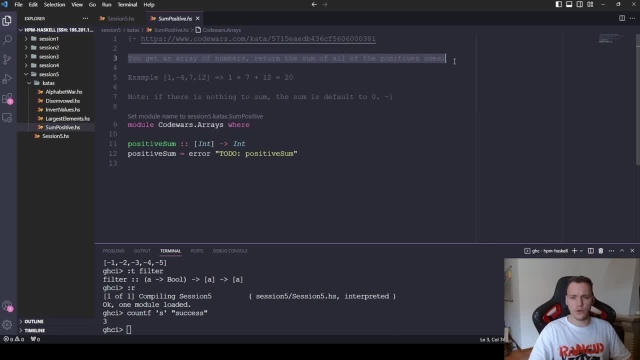 an array of numbers and return the sum of only the positive numbers. okay, if there is nothing, to some that the sum is default to zero. okay, i don't think we'll need to worry about that last time, but let's see, um, so we want, in this example, one minus 4, 7, and well, we want to. 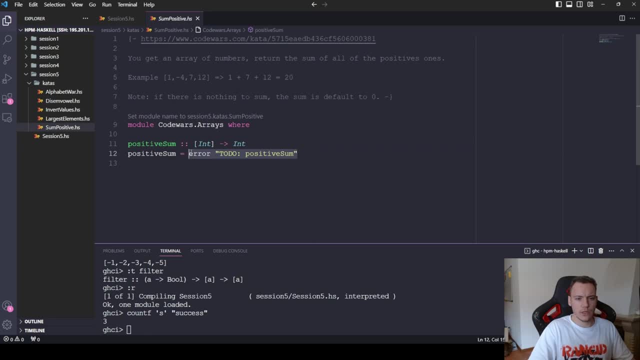 ignore 4. so basically, we can filter or we can use list comprehensions. both is both is okay. um, let's, let's covet this one. i'm not shaking it. let's go with this one. and here i we just pick it also, but let's see whether to use these well for some Buffalo, or this one instead, let's go with this one. so that's: uh, yes, let's just go with this one. so, um, okay, so let's just WHITE has some more exclusions. um, let's choose the center. so this is the Hop Shang huh, let's check if we want this one first here, let's. 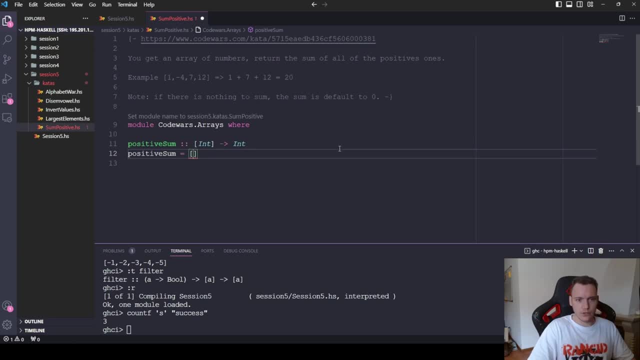 do it with list comprehension, since we started with that. so we want to create a new list of only the positive numbers, so we can use our general syntax of x, where x is taken from the list xs and it has to satisfy a predicate, and that predicate is that it has to be greater than 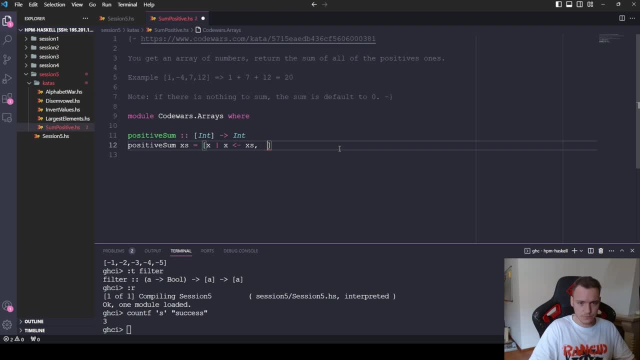 zero, so that it's a positive number. so x must be greater than zero. and now we have our filter list and all we have to do is sum it up. so if we now load, we are session four, then session five- sorry- then katas and some positive, and if we have positive, sum of an empty list. 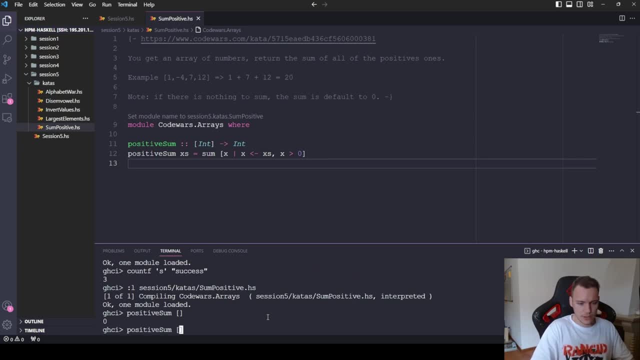 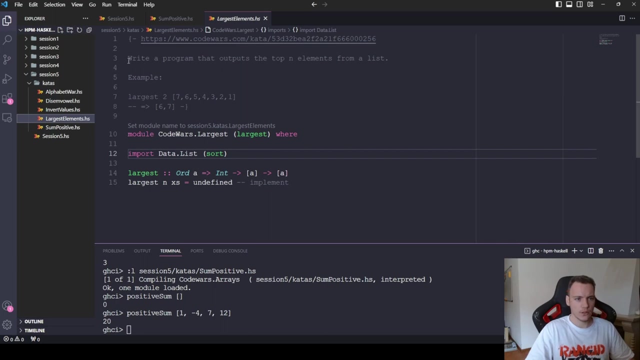 we get zero, which is correct, and if we have, let's use the example- one minus four, seven and twelve, we get 20, which is also correct. the next one will be largest elements, another simple one. so write a program that outputs the top n elements from a list. example: largest two. so 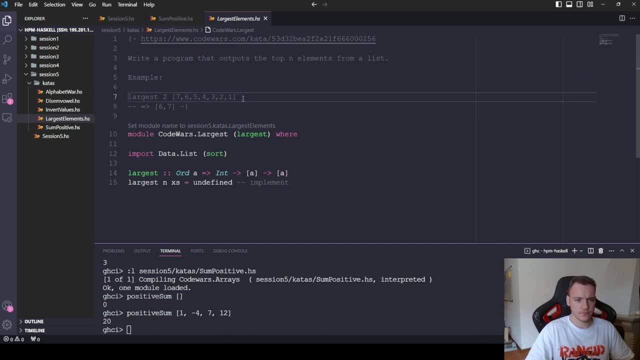 two is the n, and then a list you, and then the results should be six, seven from this list. so it seems that it also must sort it. so, because here it's seven, six, and then in the results six, seven. okay, we will say that it has to sort them as well. so 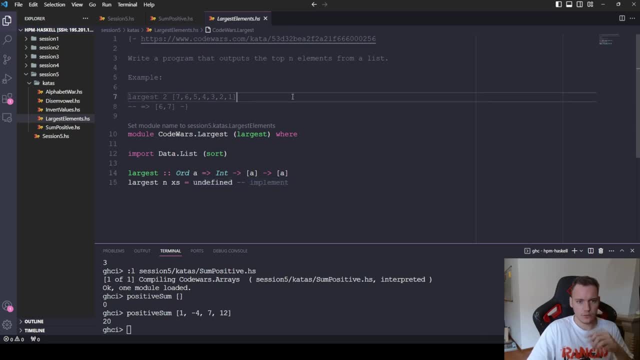 so how could we do this? if we imagine here in this example, what we first can do is we can sort the list and then we can sort the results for these sets. we have one, two, three, four, five, six, seven, and then we just want to take the last n. 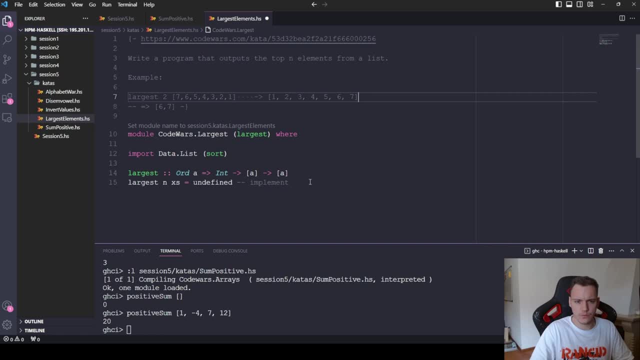 number of elements, so two, in this case six, and seven right. so so, basically, this will be a combination of sort applied to the list xs, and then we can compose the result as one, and so we have the result xs. then we can deal with the tightly and then we can decide which format, Gavin, you want to use. 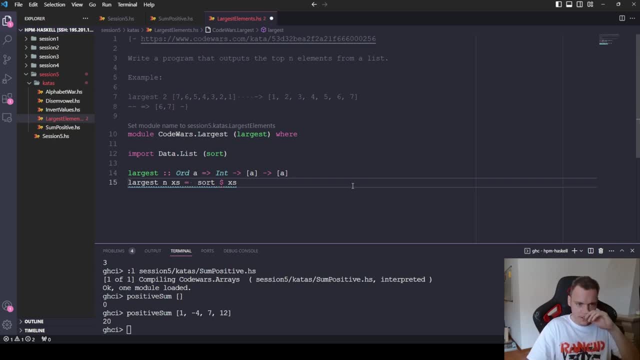 you, Una, you know, you know I could use any format and then check, as in our case. however, this function with the, with the drop function, right, so we want to drop all elements except the last n and the. the trick is then: how many elements do we need to drop if we know n and? 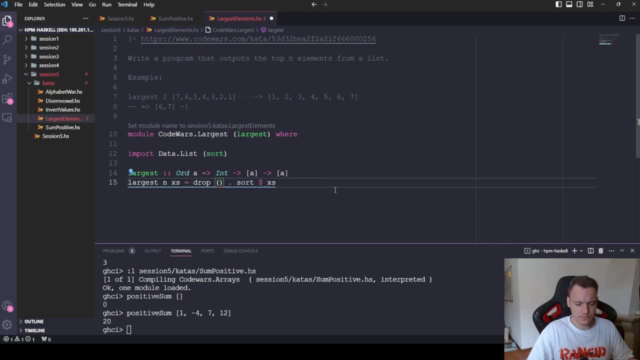 obviously also. we know the list, so we know the length of the list. so to drop: in this case we want to drop five elements. right, the length of the list is seven and the n is two, right. so seven minus two, the length of the list minus n, is the number of elements we want to drop. right. so length: 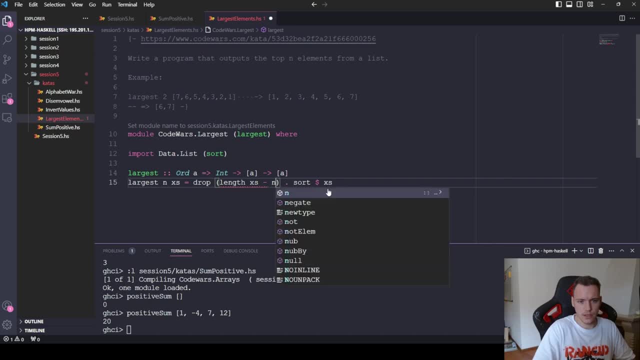 of xs minus n is the number of elements we want to drop. and now we have to load largest elements and we can test with largest. so we can use this example: largest two, and now we get back six, seven. so we could have done this in a different way, of course, 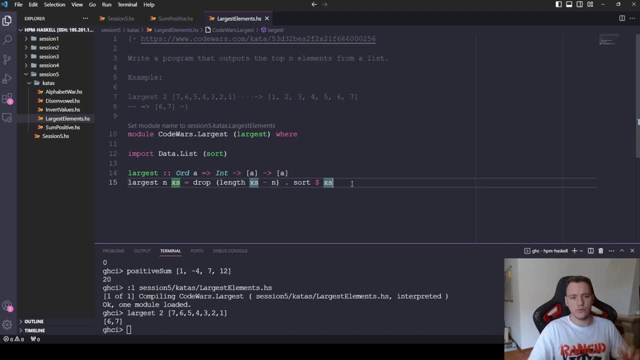 like we could sort it, then reverse it to get the highest elements in the front and then, instead of drop, use just take n, but that would that would then give us back the results seven, six in this case. so we would have to reverse that final list again. 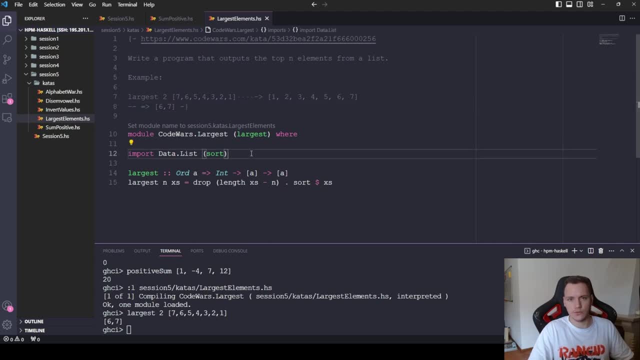 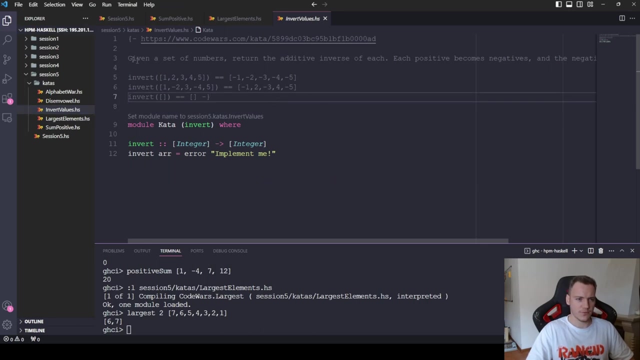 anyway, always a lot of things, a lot of ways to do the same thing. in this case, this is our solution for now. moving on to the next kata invert values. okay, yeah, the this is going to be the same as i gave in the example. okay, yeah, the this is going to be the same as i gave in the example. 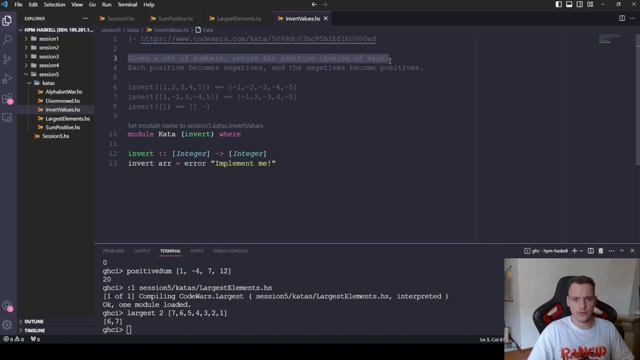 okay, we're going to reverse that and i'm gonna call it here. so now remember: left null, we have aね and right null and it should represent the result and 不是. all the numbers here will be negative. yeah, so we have like we have zero saved and only one negative one will be negative for the map function, but okay. 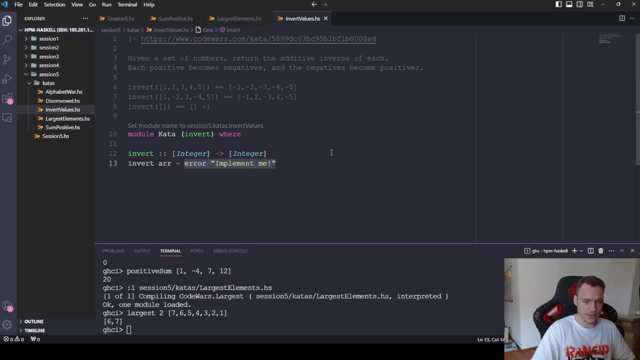 okay. so we basically wrote this function at the start of the session and we just want to map the negate function. that will negate a number, so if it's positive it will be negative, if it's negative it will turn into positive. we map the negate to array and we can also use eta reduction. 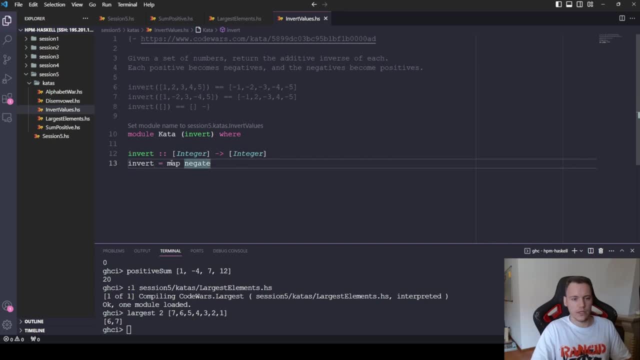 we don't need array here, so we can define invert as just the function map negate to the argument it receives. and if we load session five, cutters invert in oh, invert values and then we invert this example correct. this one is more interesting since it contains both. 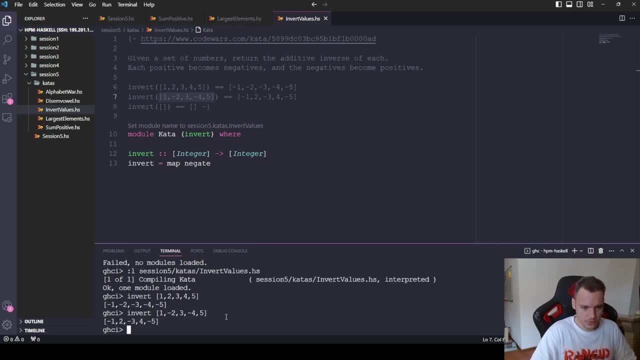 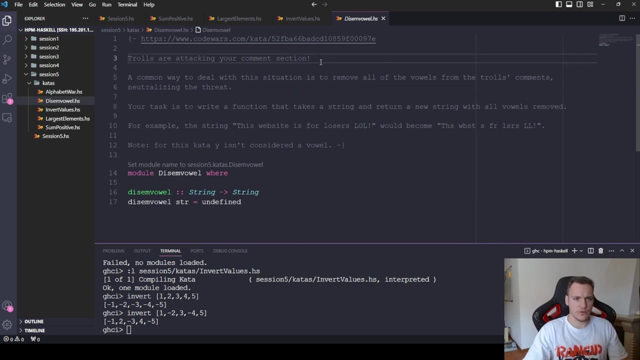 positive and negative. so one becomes minus one, minus two becomes two, and so on. so you see, the negate is applied to each argument and a new list is formed. the next one will be a bit more interesting. it's called disemvowel and it says the trolls are attacking your comment section. 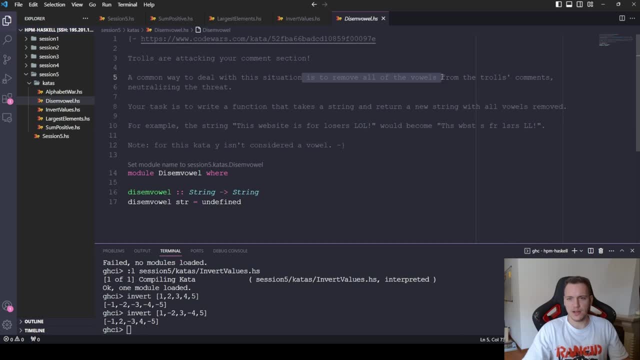 so the what we want to do is remove all the vowels from the troll's comments. okay, so we need to write a function that takes a string and returns a new string with all vowels removed, in other words, filters, a list of characters, a string. so, for example, this website is for losers. 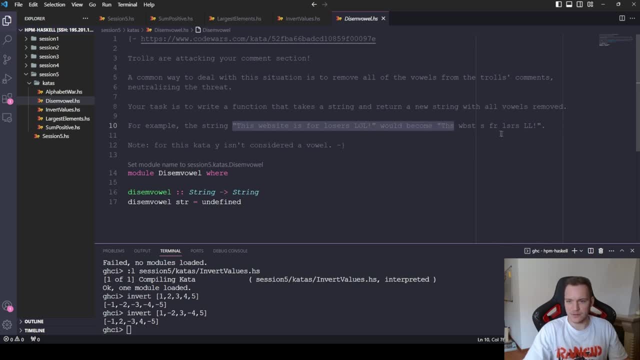 lol. for this data, y isn't considered a vowel. okay, so we can see. we go from this list to this list, which is basically the same, except some characters have been filtered out. so obviously we can make use of our higher order function filter. we can also do it with list comprehension, but since we 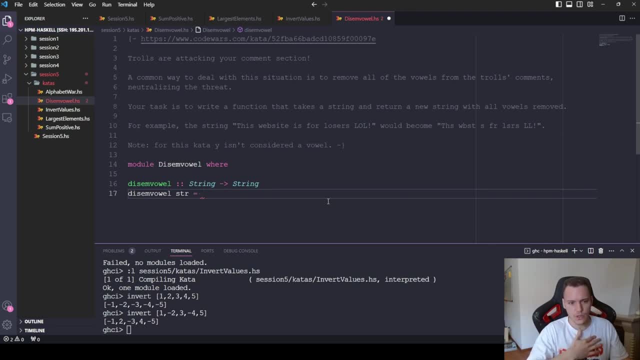 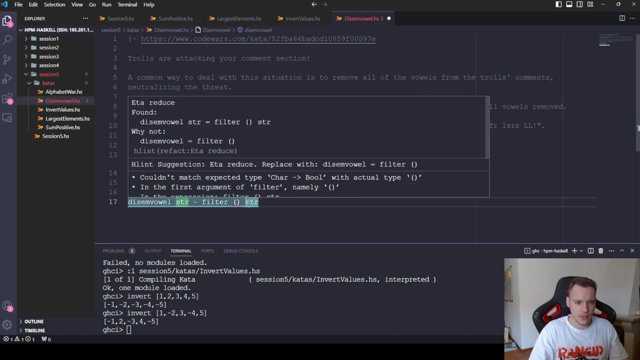 we already use that. let's use filter here. so we will want to apply the filter function and then we we have to apply some function and apply it to our string, and we need to. we need to define this function. so our function should filter out vowels. all right, so we can. 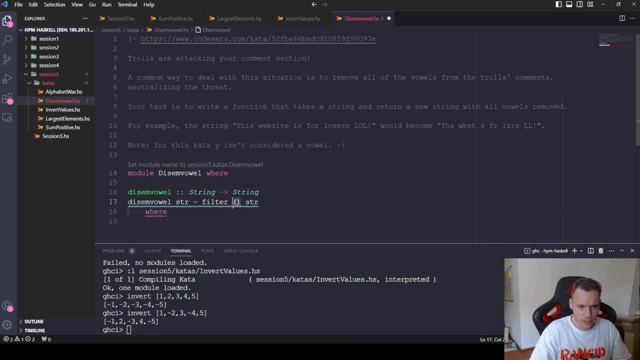 define it here in the where and we'll call it so we. we basically want to filter for, not vowels, right? if it's a vowel, we want it filtered out. if it's not a vowel, then it stays. so we can call this function is not vowel, and if not vowel will be defined here. it will accept a character also. we. 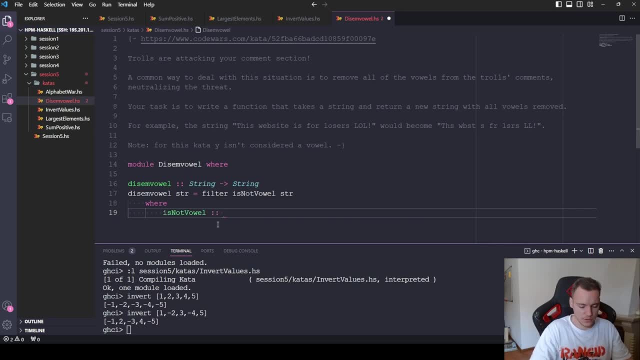 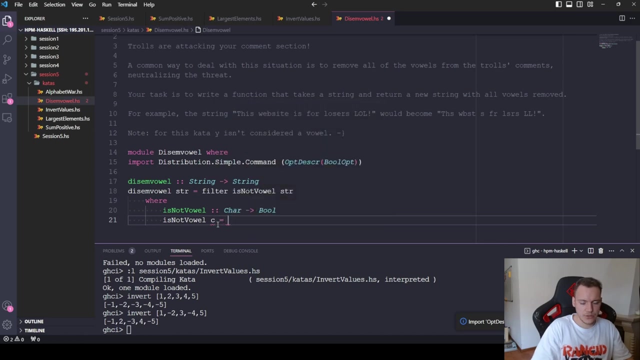 can write type signatures for functions in the where clause as well. right, so we can say it accepts a character- we know that it must return a boolean, since we're going to use it with the filter function and is not vowel- then accepts a character, character c and then. 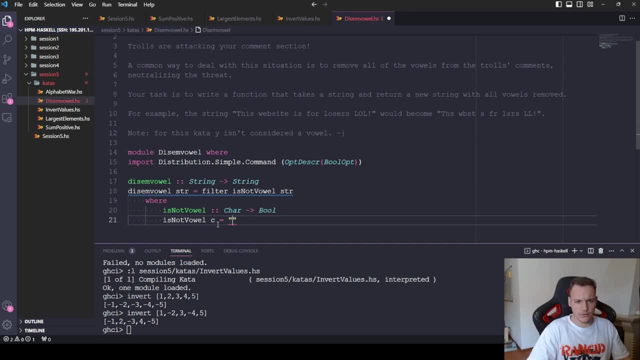 uh, what do we want to check that it's not a vowel. so the vowels are a, e, i, o, u. right, those are the vowels. y is not considered a vowel. i didn't really know it. it is a vowel, uh, but anyway, a, e, i, o, u, those are the vowels. so we want to check that. this character. 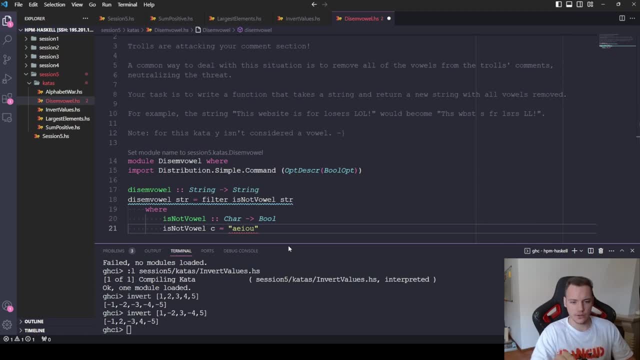 is not, is not in this list, right? it's not any of these characters. so we saw the function lm, haskell, which checks whether an element is exists in a list, and here we want to use not lm, which is the same function, but negated, right? so we want to check that c is not an element of of the vowels. 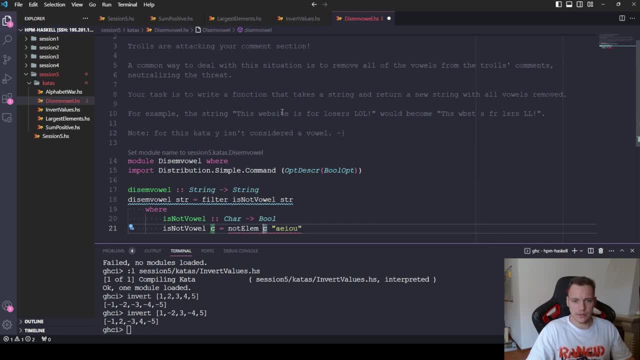 and we have to deal with case. uh right, because we could have a vowel that's capitalized and then it will not. oh well, we can either deal with case in two ways we can. we can spell the vowels here in capital case as well. so now this: this is okay, um. 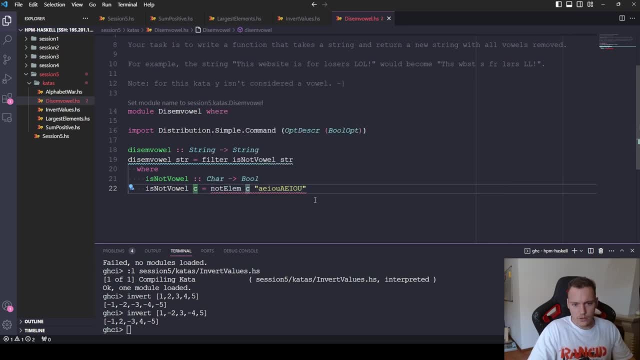 okay, we can refactor it, uh. or we can say: we can say two lower c, compose, compose these two and then apply it to our vowel list. i will do it this way, okay. yeah, so it's saying we can write it in a different way, basically two lower c and then. 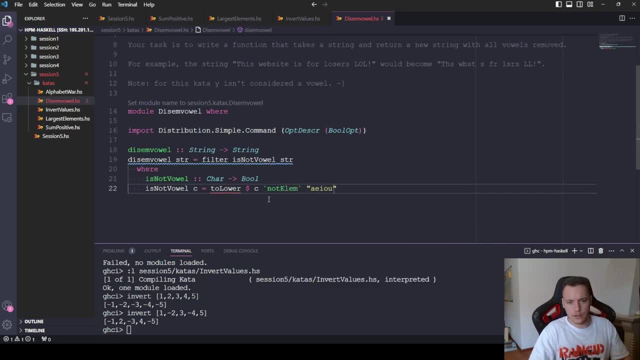 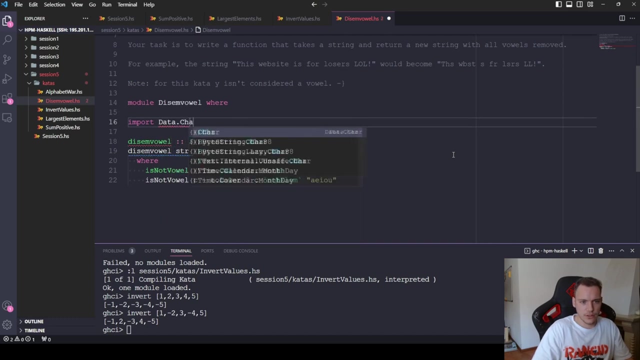 using our infix operator, not lm. um, um variable not in scope too lower, so two lower is actually. oh, this got filled in right, because i auto completed something we don't need. that um two lower is actually in this package called datajar, so we can import this function. um two lower is actually in this package called datajar, so we can import this function. it simply accepts a character and puts it into lower case type. and then we can import a goddamn input parameter and variable out autres random variables to implement. v أيo, this got filled in right, because i have to completed something we don't need. that um too lower is actually in this package called datachar, so we can import this function. it's simply accepts a character and puts it into lower case. finds this input quality here. 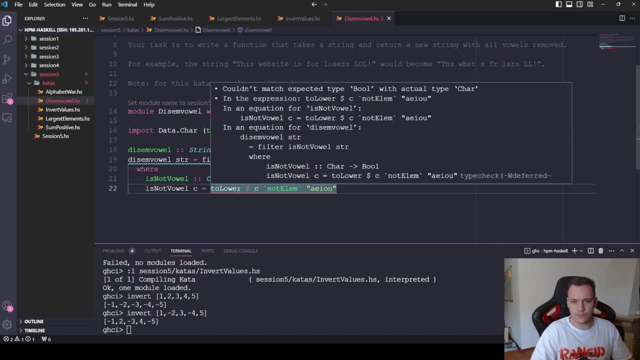 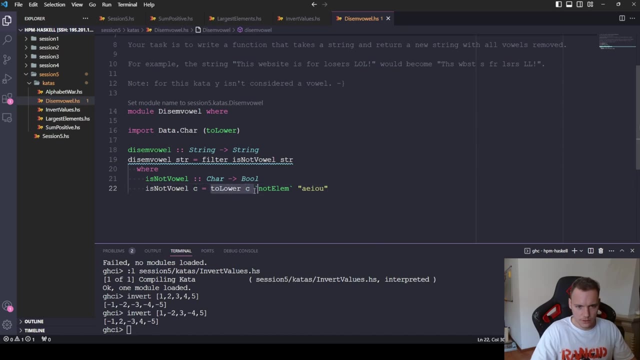 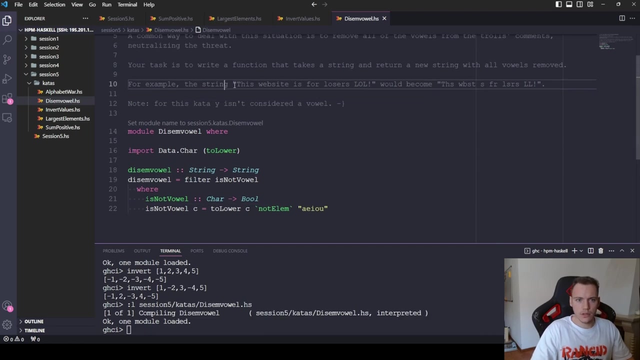 a character and puts it into lowercase. so something is wrong here. I guess the application operator is not needed here. so to lower C is not an element of the lowercase vowels. also, here we can remove string on both sides, and that should be it, so we can load this unvowel and we can test it with this. so this: 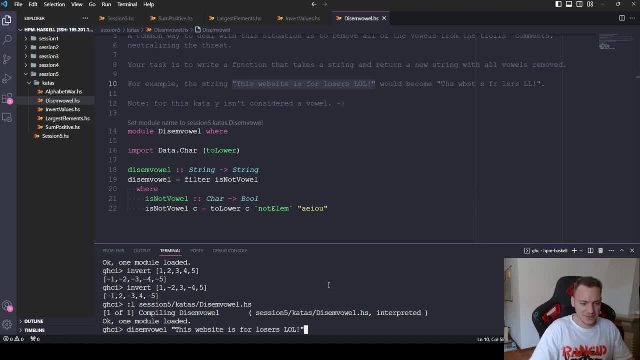 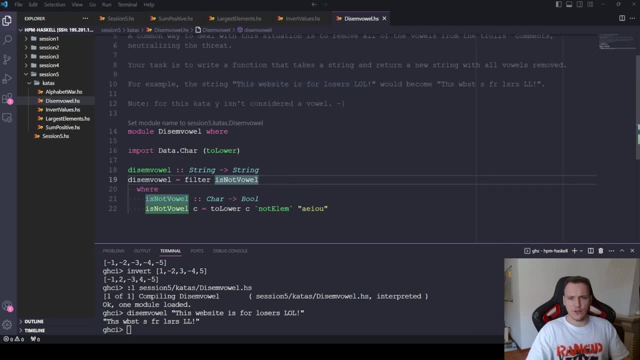 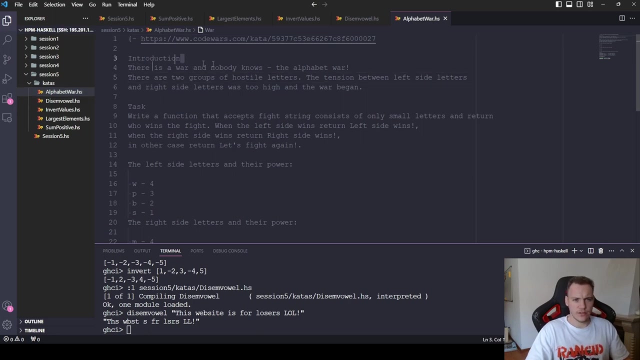 unvowel. this website is for losers and this website is for losers too, works fine. okay, it's time for our last kata for this session, called alphabet war, and it says there is a war and nobody knows it's the alphabet war. there are two groups of hostile letters. left side: 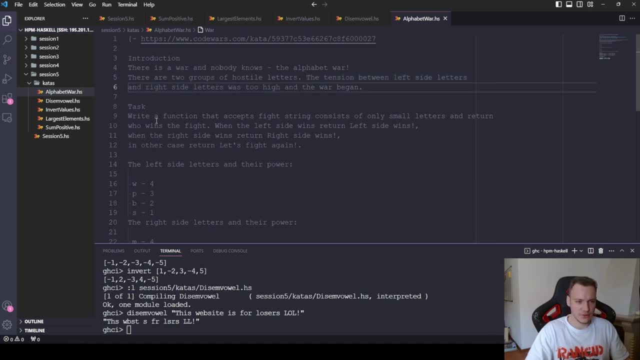 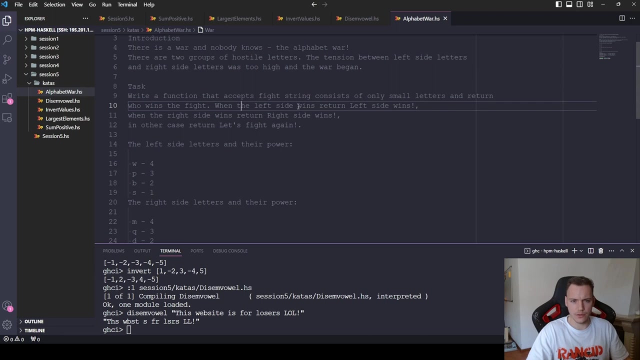 letters and the right side letters and we need to write a function that accepts fight string consisting of only small letters and returns who wins the fight. so we accept a string and we return a string. so when the left side wins, return left side wins, otherwise we return right side wins. or. 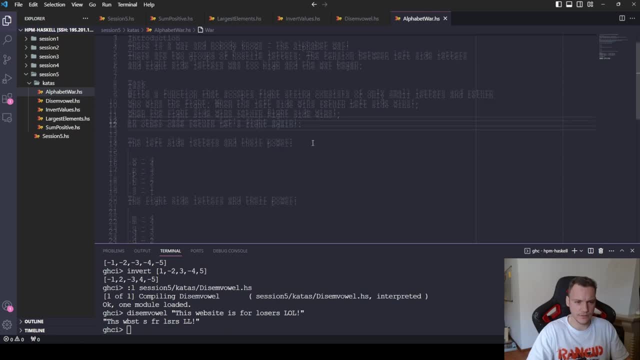 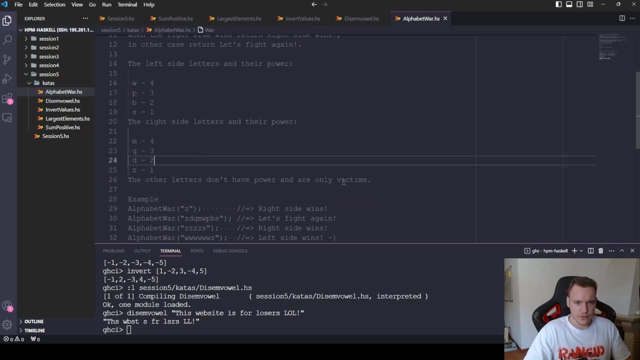 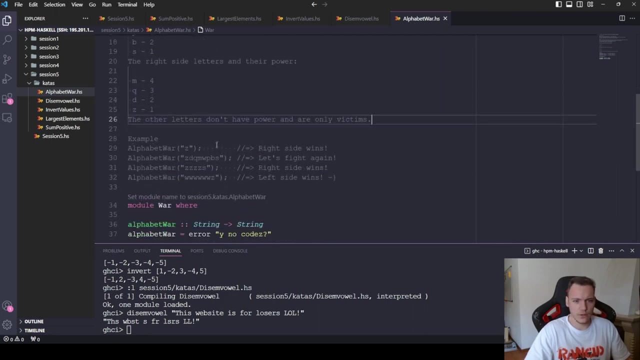 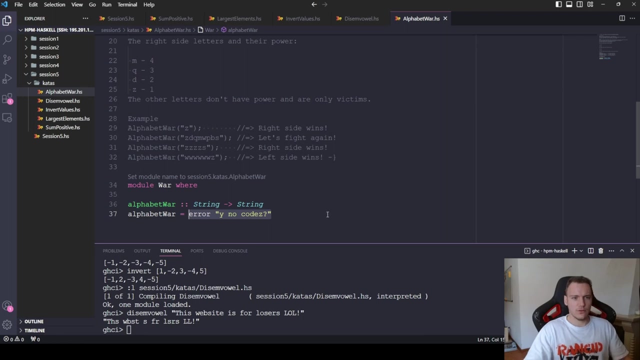 it's. if it's a tie, then we return. let's fight again, okay. left side letters and their powers. right side letters and their powers. the other letters don't have power, and only victims. so i guess their power is zero, and okay. so what we could do is write a function that maps a character to a value, to an integer value. 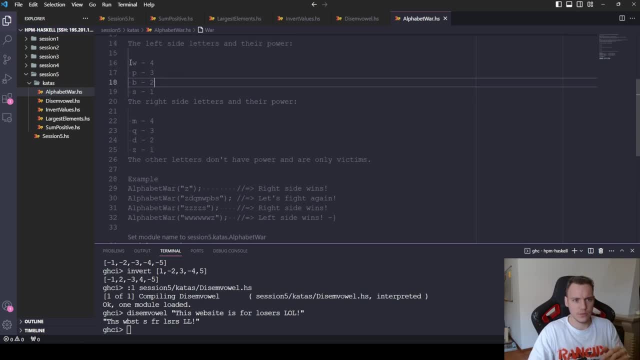 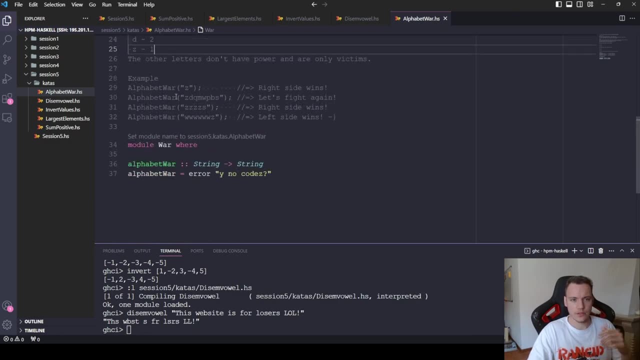 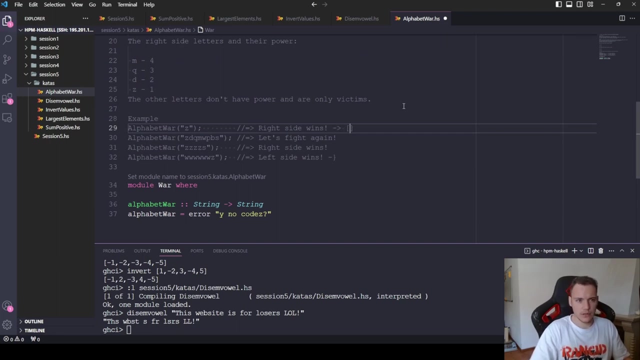 such as this, so we can use, for example, minus for the left side and plus for the right side. we will then create a new list. so, for example, this list z would, after mapping our function, z has one, so it will become a list of one. in this case, it would be like z is one. 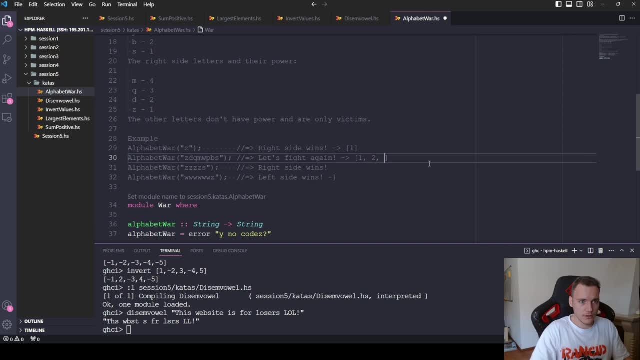 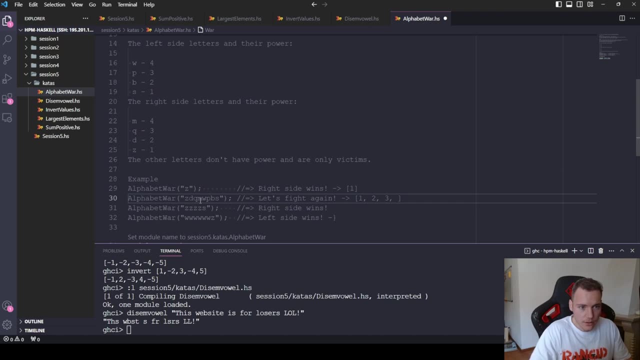 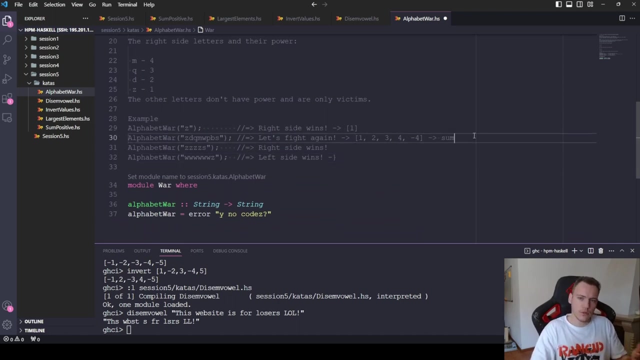 then d is two, then q is three, but give me a left side, so it's gotten. it's d the left side and u is two, it's d the top. okay, d is four, but m is okay four, and then the left side, w is four, so and left side will be minus four. okay, and then if we 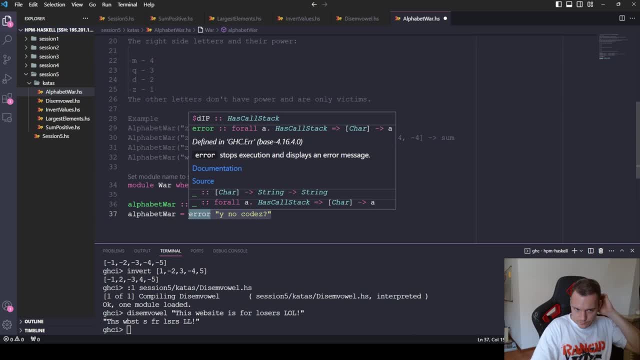 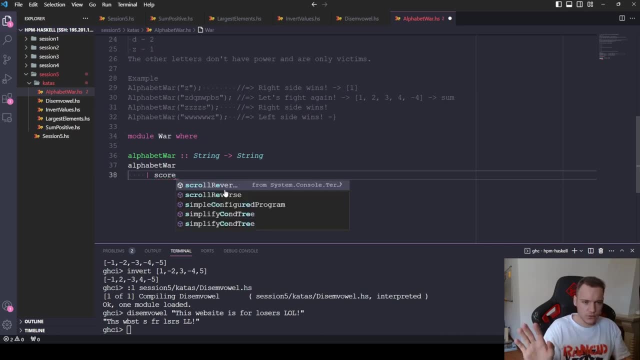 if we then sum that up, we get the score and we can decide which side wins, right. so so we can write the like the high level, with a guarded equation. we will have some score that will calculate greater than zero. then we will say: so, what do we say right side? right side will be positive. so 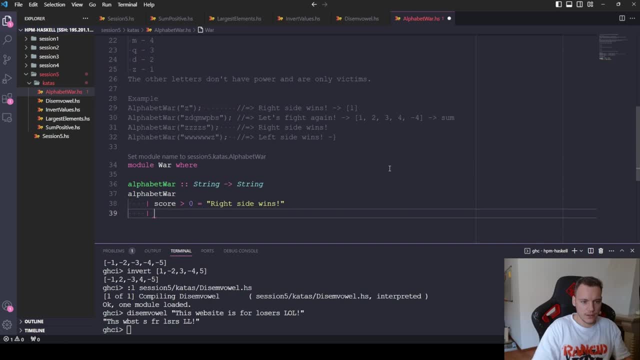 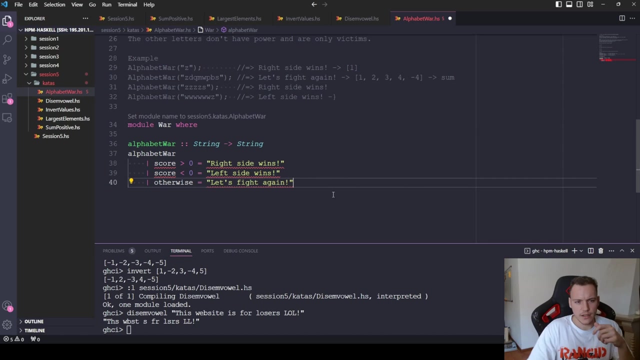 right side wins, okay. if the score is less than zero, then we will say left side wins and otherwise we will say let's write again. okay. so that's like our how, how higher level, how our function should work, and then we need to say where score is going to be. so the sum, the sum of 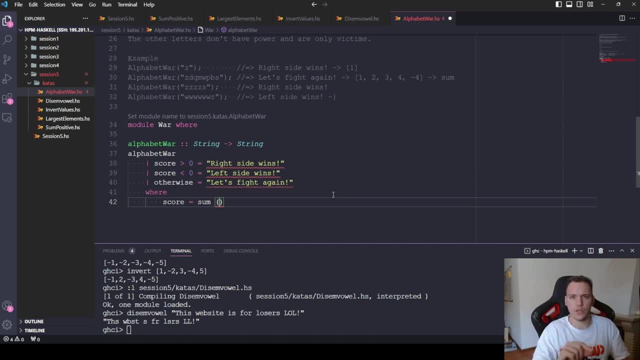 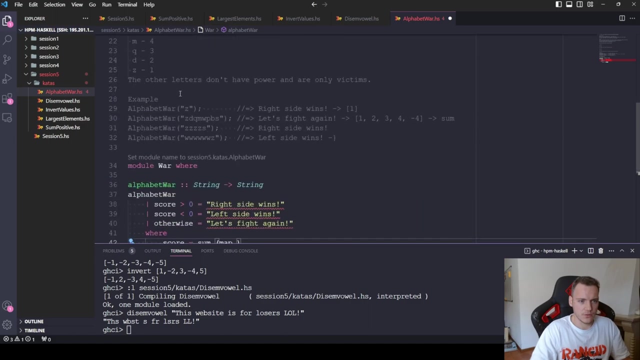 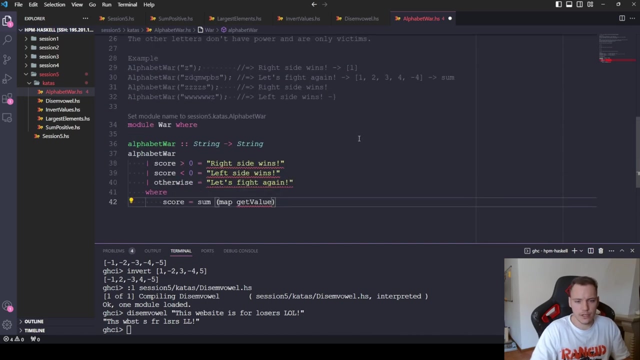 the score, our new list that we get by mapping our new function, which we also didn't define yet. so sum applied to this new list that we'll get by mapping the- what should we call this functions. for example, get value, get value from character applied to, so this: 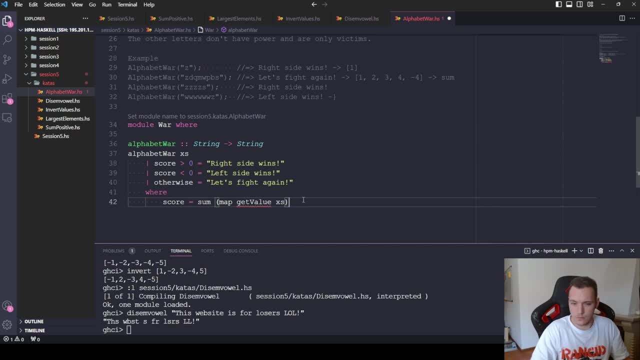 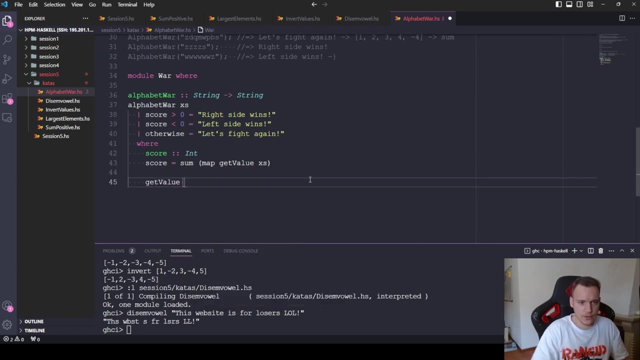 x, s that we get as the string. this looks okay, and so, finally, score should be just an integer value. what we don't have is the get value function, and get value is a function that so it will be mapped to a list of characters, so it will be applied to each character. 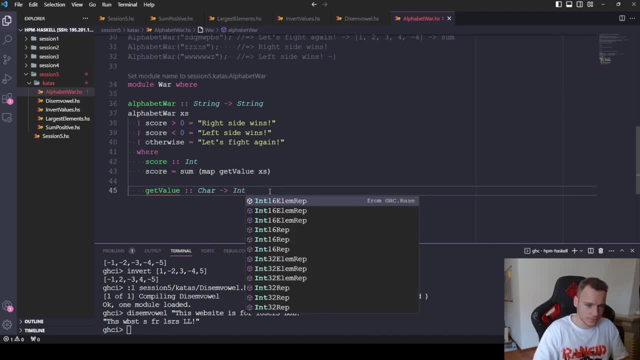 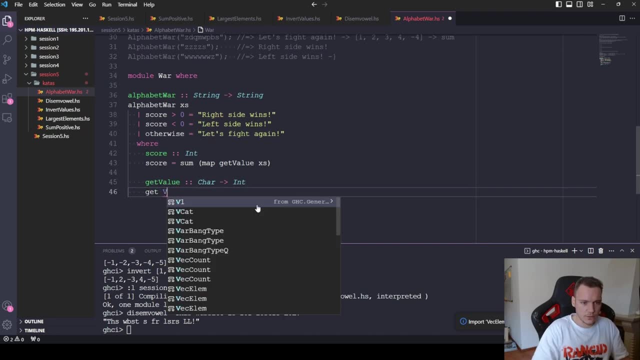 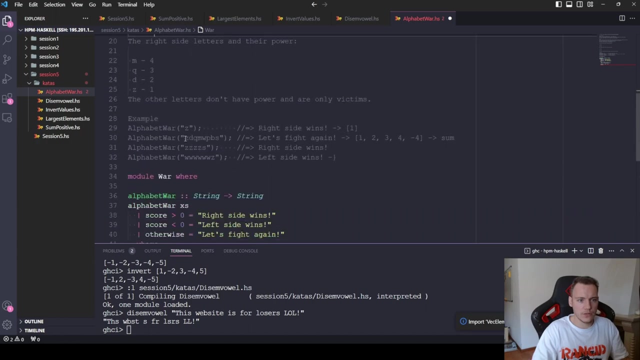 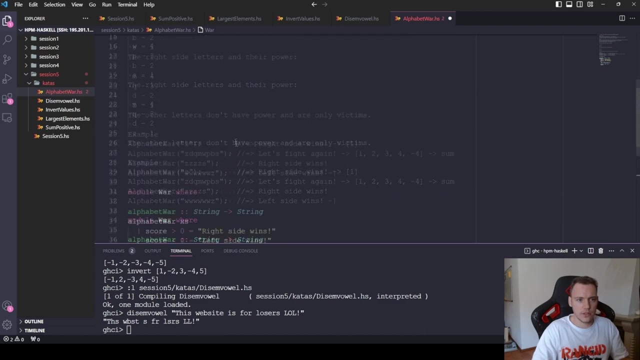 to accept the character and it will return an integer right. and now, how do we define that? well, since these are just arbitrary values- four, three, two, one- we don't have much choice but to list them all out, right? so we just have to list each character one by one and assign. 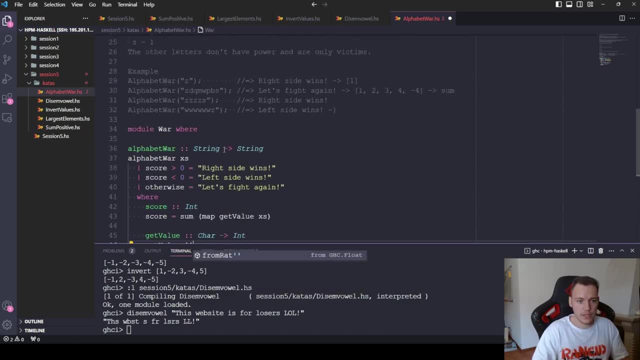 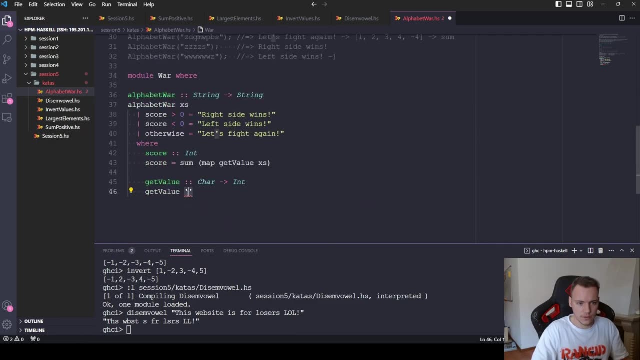 it a value, so we can use pattern matching here. let's do the left side first. so it's going to go something like this: so get value w is going to be left side. we said minus, so minus four. then get value e, b and s, so there will be minus three, minus two, minus one.